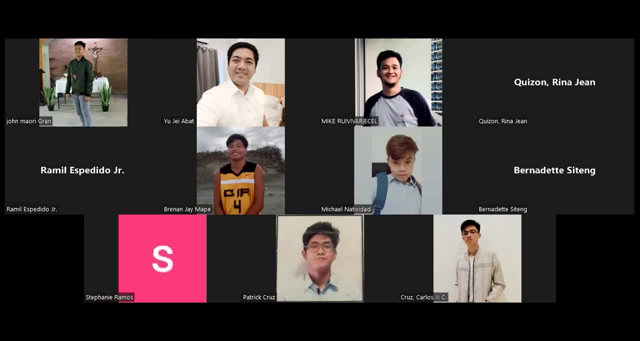 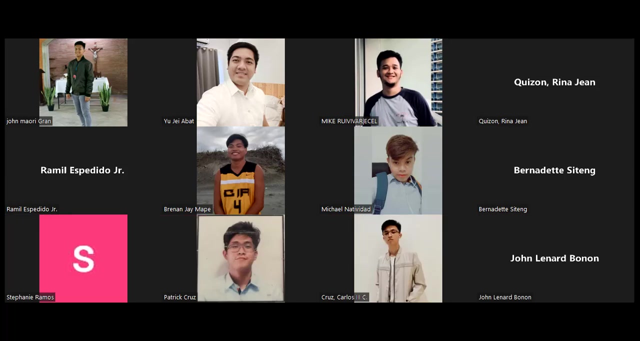 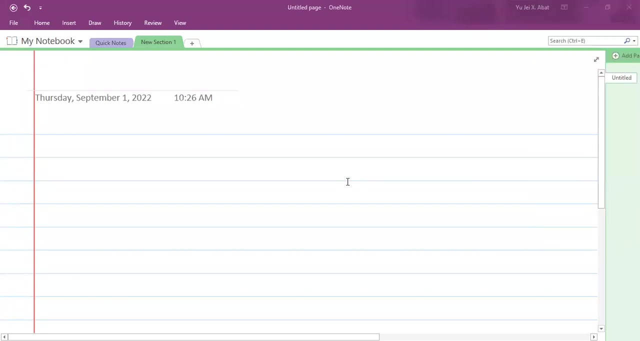 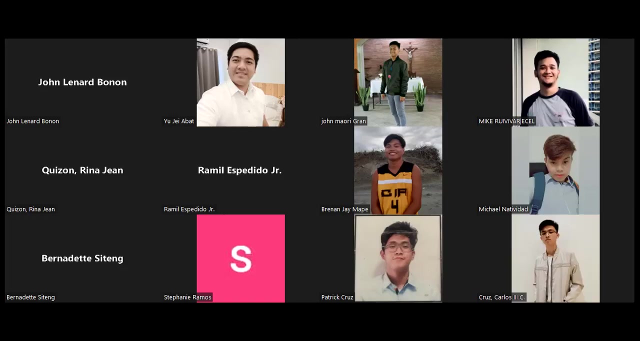 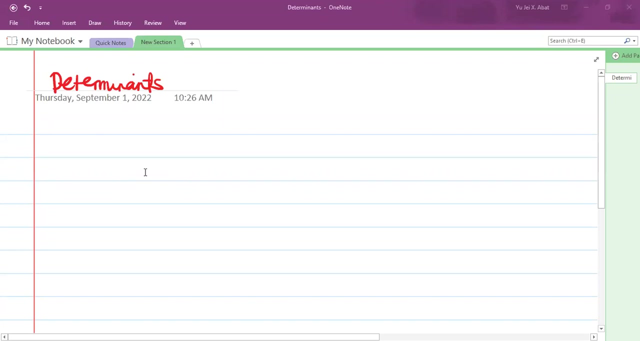 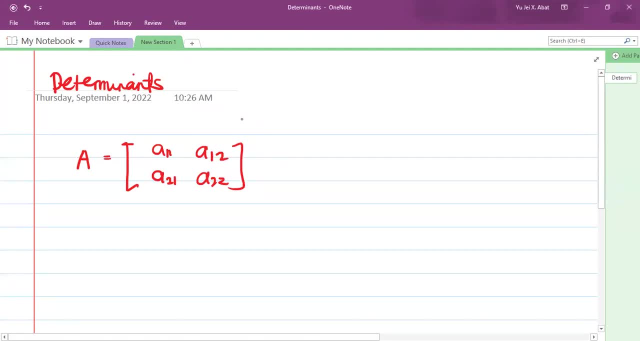 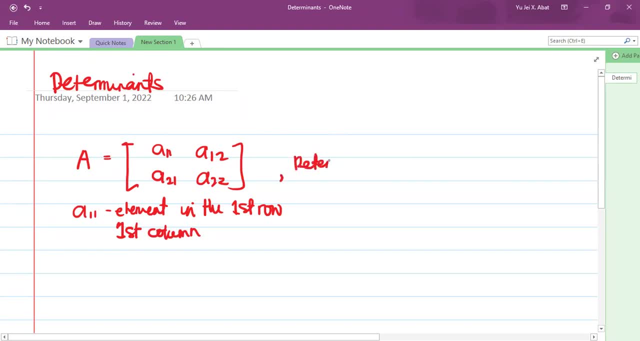 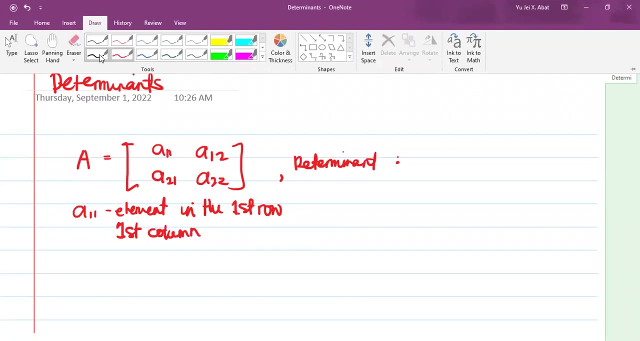 Now, the definition of determinant is this. If we want to get the determinant, is a matrix we want to get a determinant of certain matrix it will mangyari okay so or yeah 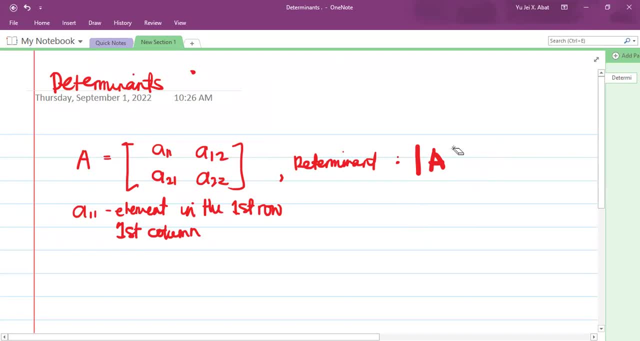 so anyway of the matrix a that means determinant for example 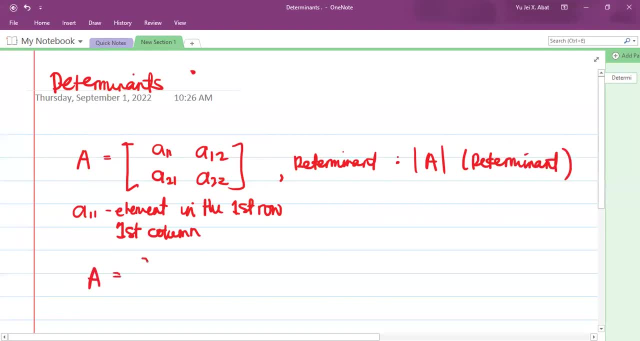 if we wish to find the determinant 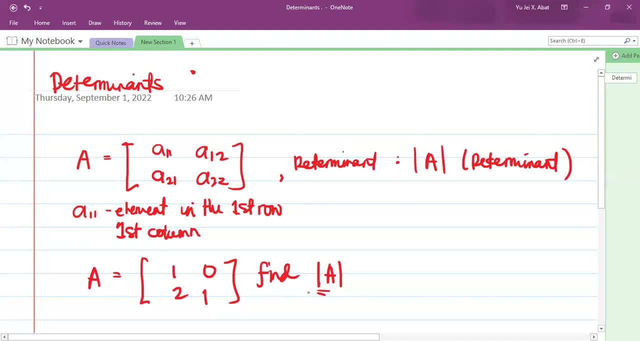 is ayan yung pakikita nating symbol okay 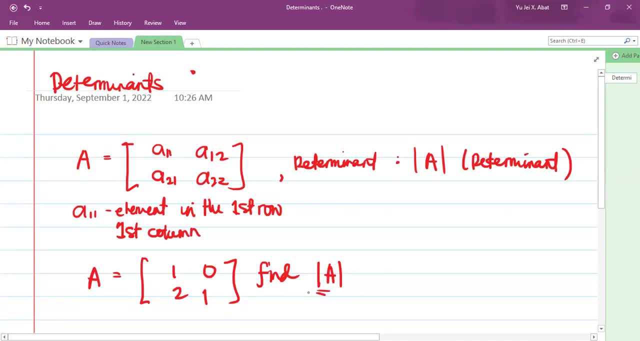 so determinants are very useful when it comes to solving systems of linear equations solving unknowns and they are some some of these steps are only itong determinant is part lang ng solution para makuha yung mga unknown values yung maraming gamit yan so that's the determinant 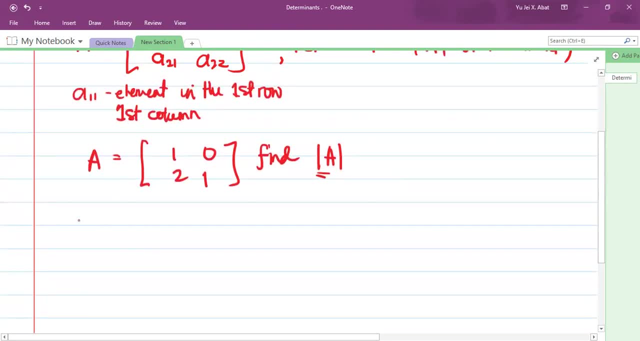 now paano ba yung definition ng determinant so if you want to get the determinant it's actually 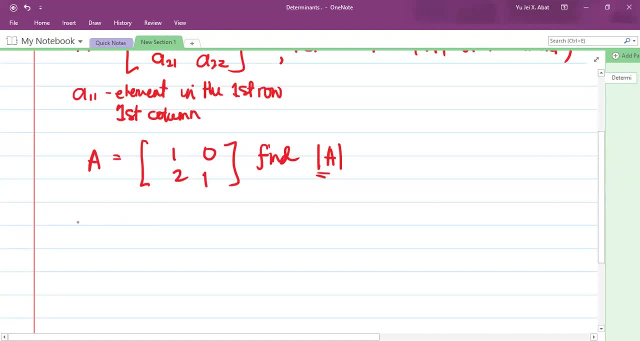 this is one no so if you have the matrix a na 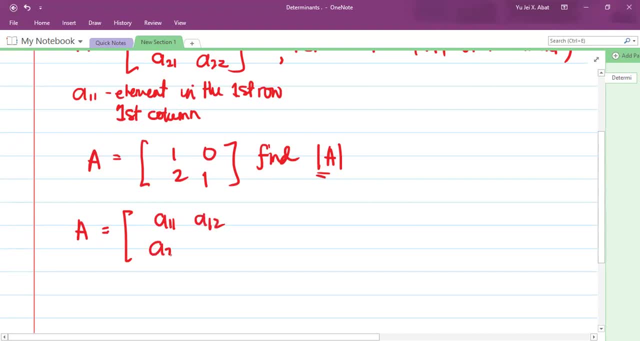 again a one one a one two okay lang yung voice ko guys okay lang okay so for example meron tayong ganyan na na na matrix 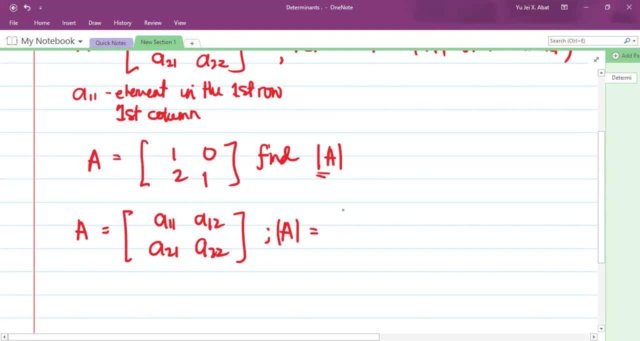 so pag ginamit natin or hinanap natin yung matrix a okay yung determinant niya that would be okay a one one no sorry 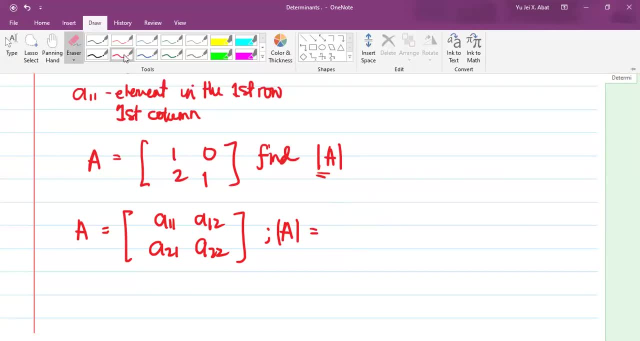 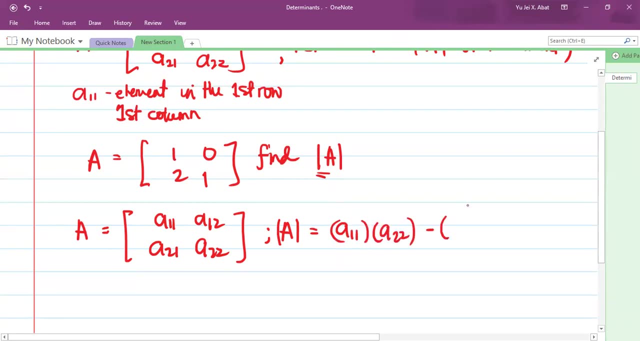 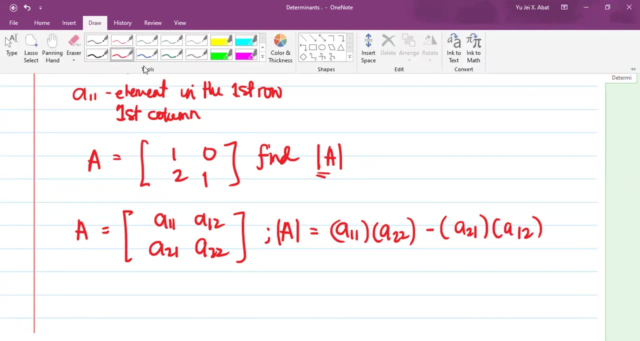 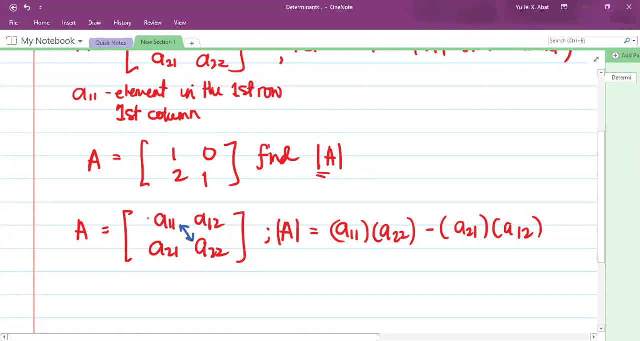 that would be a one one times a two two minus a two one times a one two so parang yung pag kuha ng determinant kasi in a two by two it's actually the summation or the product of this diagonal ito muna minus yung product nung other diagonal minus ito naman 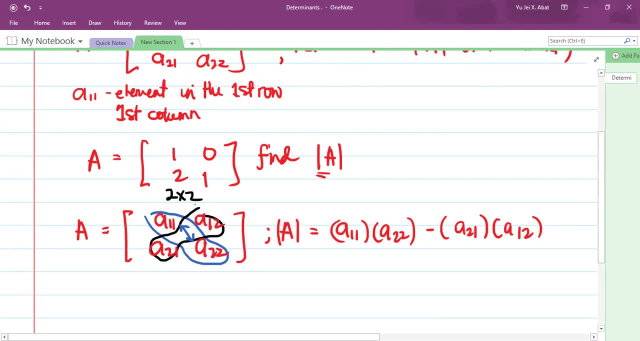 okay that's for a two by two matrix 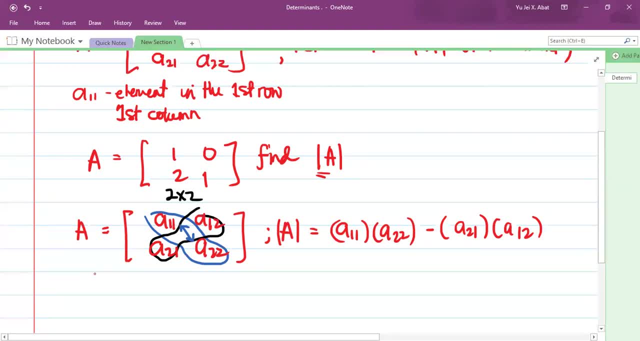 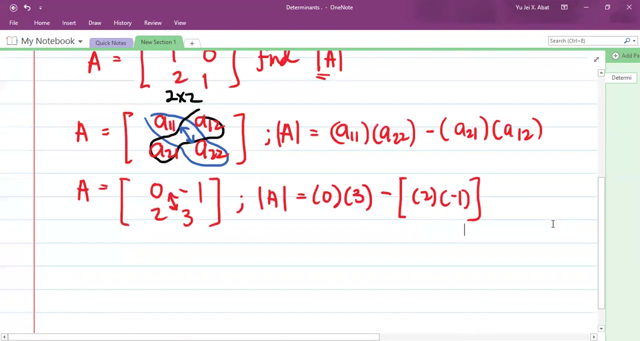 no so for example meron tayong matrix matrix a zero negative one two three if we're going to calculate the determinant of that matrix that would be zero times three dahil ito yun okay okay and then minus laging minus no laging minus the other diagonal the product of the other diagonal that is two times negative one okay so pag sinov natin yan obviously this becomes zero minus 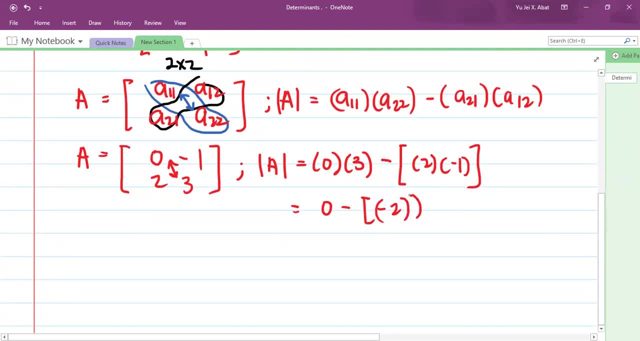 that is negative two dahil negative two negative one times two is negative two so and take note 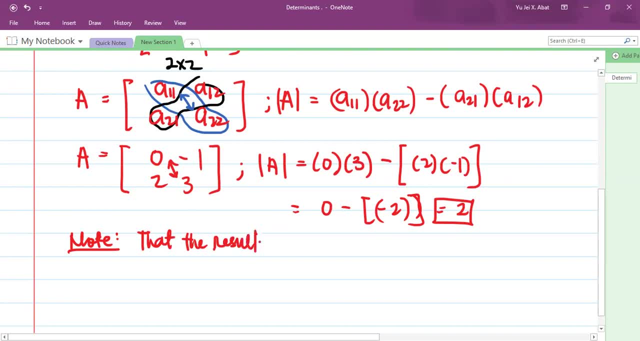 that the result of a determinant of a determinant is always what a scalar quantity 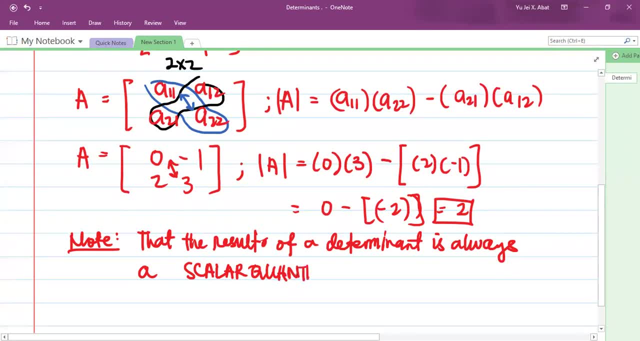 so ibig sabihin na a scalar quantity number sya so meaning constant number Okay? Understood? Yes, coach. So another one, if you're going to try. 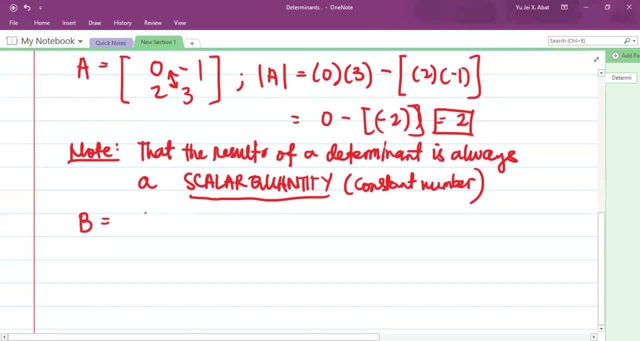 By the way, class, yung mga kinukuha lang natin dito na determinant is square matrix. Again, pag sinabi natin square matrix, same row versus same column. So we have negative 1, 2, negative 10, 1. So if you wish to find the determinant of B, that would be negative 1 times 1. So nasan nang galing yun? Ito. 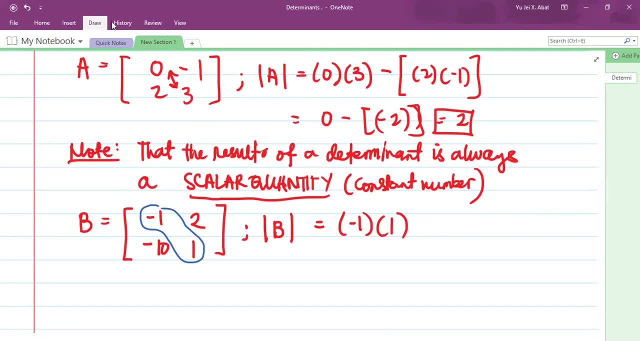 Yung diagonal na yan. Then minus the product of the other diagonal. Minus, yun lagi yung formula. Yung minus the product of the other diagonal. 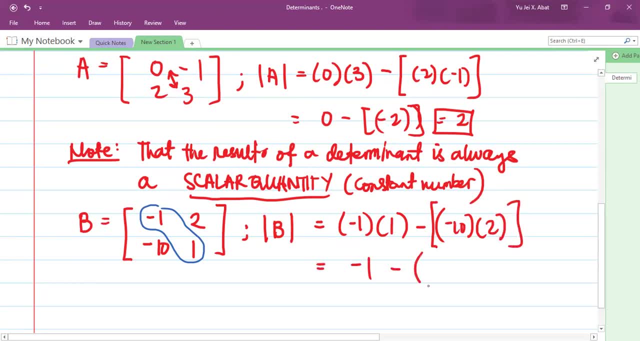 So negative 1 times 1 is negative 1 minus negative 10 times 2 is negative 20. So we have negative 1 plus 20, that's 19. 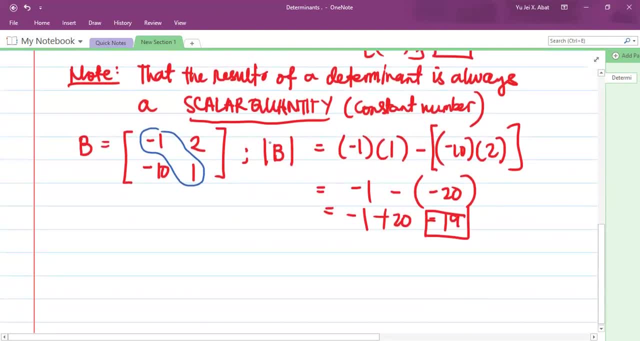 Okay? Yan ang determinant ng 2 by 2 matrix. 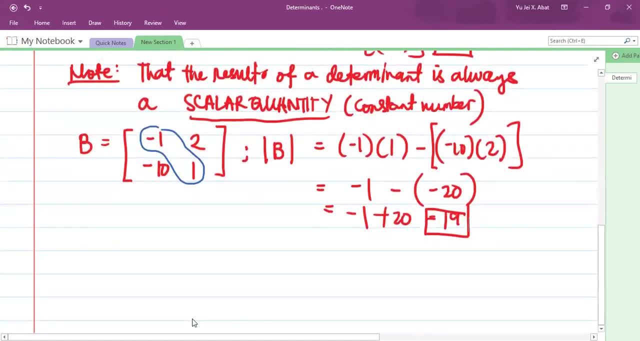 When it comes to 3 by 3 matrix, for example. Okay, so medyo higher naman tayo. 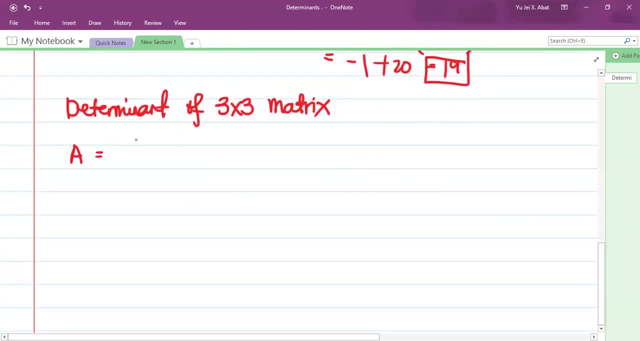 So suppose we have a matrix, A11, A12, A13, A21, A22, A23. So we have A31, A32, A33. For example, yan yung matrix natin, 3 by 3 matrix. Now to get the determinant, this would happen. Okay? Okay? To get the determinant. To get the determinant, I will be first deriving this. 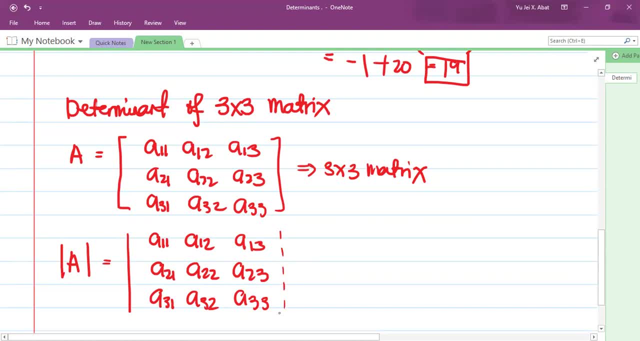 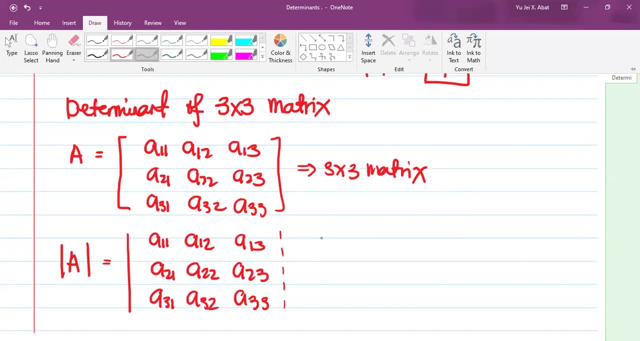 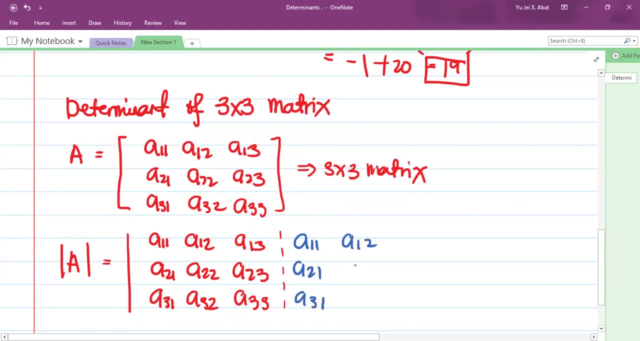 And I will copy the first two columns of the determinant. Okay? Okay? Okay? Okay? Okay? Okay? So that would be A11, A21, A31, A12, A22, and A32. Okay? So yun muna yung gagawin ko dyan, guys. Okay? Wait lang. Yan. 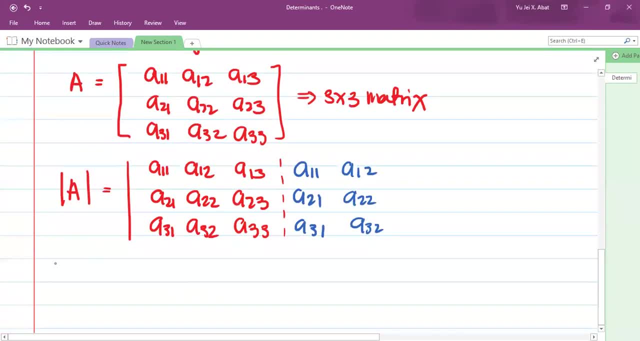 So in that, yung gagawin ko, I will get the summation of the products of the diagonals. 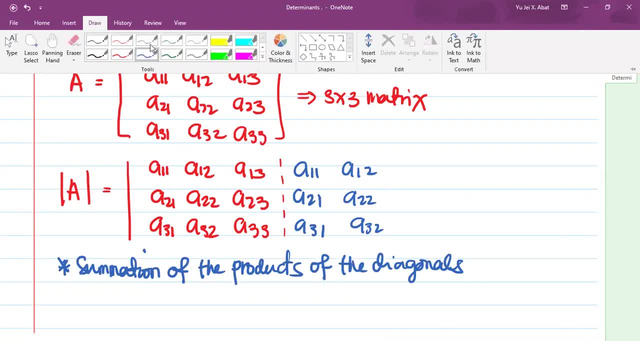 So ano yung summation ng products ng diagonal? So una kong diagonal is ganito. 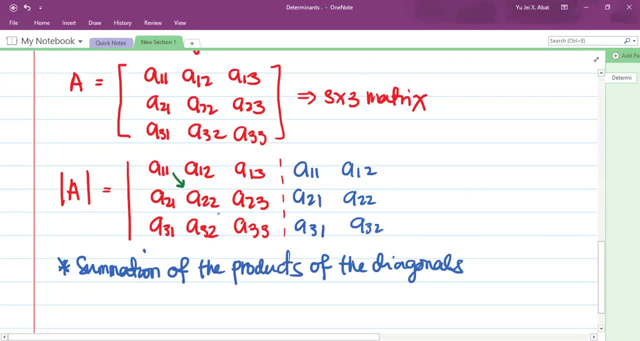 I have the first diagonal, A11 times A22 times A33. Okay? I have the second diagonal. 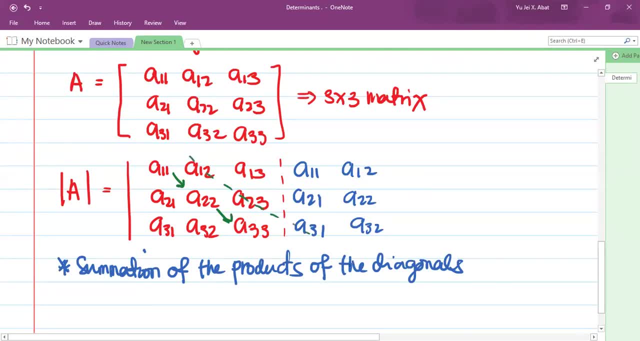 I have the third diagonal, A12, A22, A23, and A31. I have the third diagonal, A13, A21, and then A32. Okay? 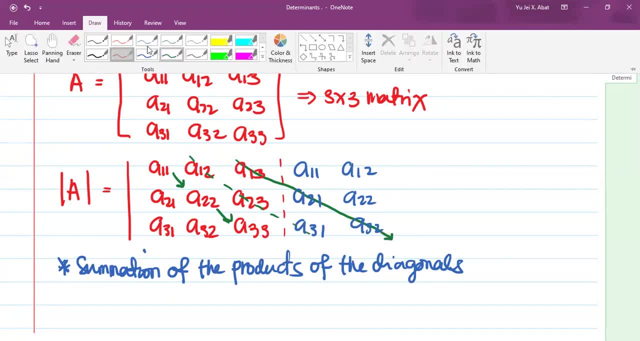 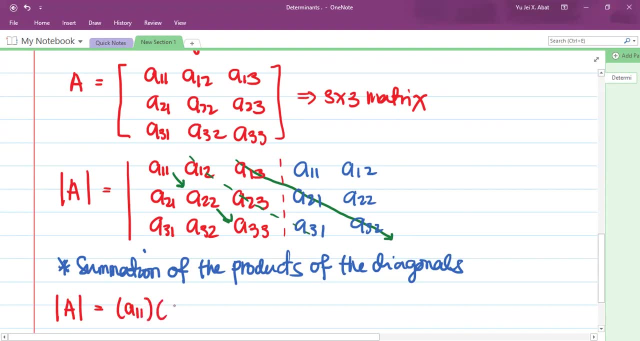 So yun yung magiging formula natin. So if you're going to get that, so you have determinant of A, that would be A11 times A22, the first diagonal, and A33. Summation of the products. So ibig sabihin, summation ng products nila. So plus the second diagonal, which is this one, so you have A12, A23, A31 plus, again, the diagonals, the third diagonal in this case. 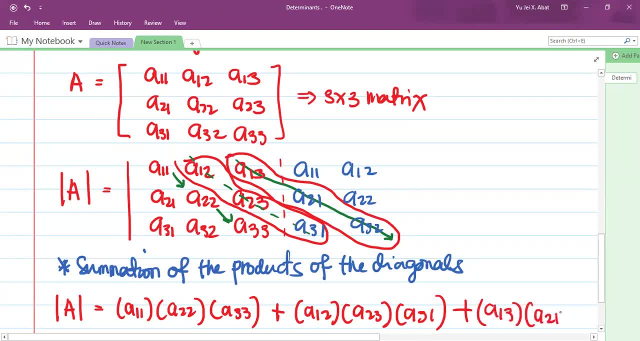 So we have A13, A21, and then A32. 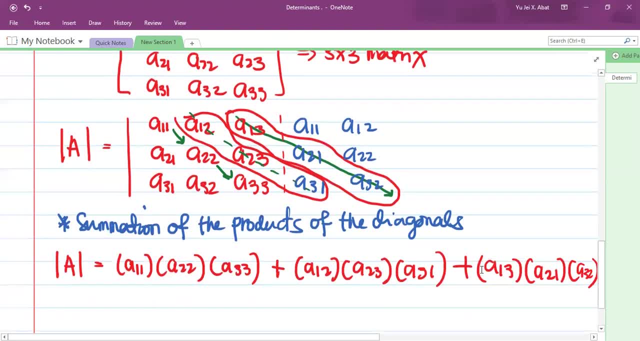 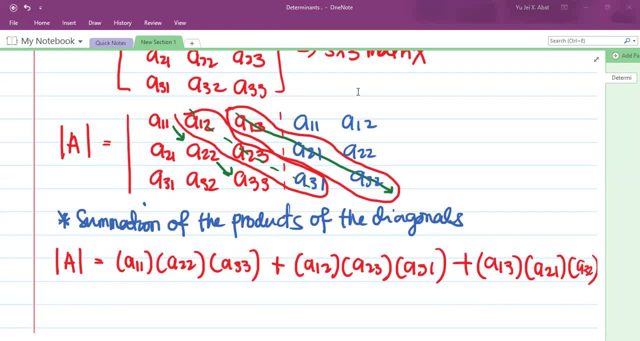 And then, syempre, na-clear mo na lahat yung tatong diagonal, no? So ngayon, ano naman ang sunod? Yung susunod naman yung other diagonal. Yun. Sa biyahe. Yung susunod naman yung other diagonal. 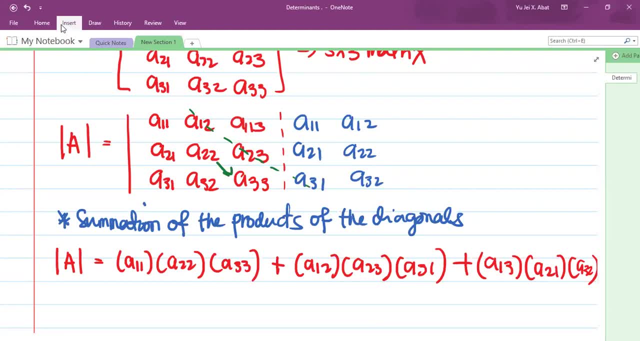 Okay, so A13 to. 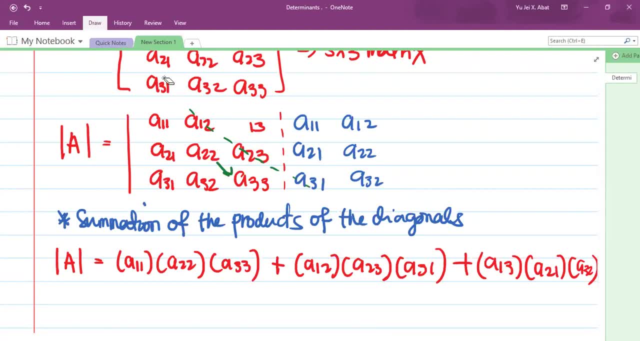 Erase ko lang. Para mas malinis tignan. Ayan. 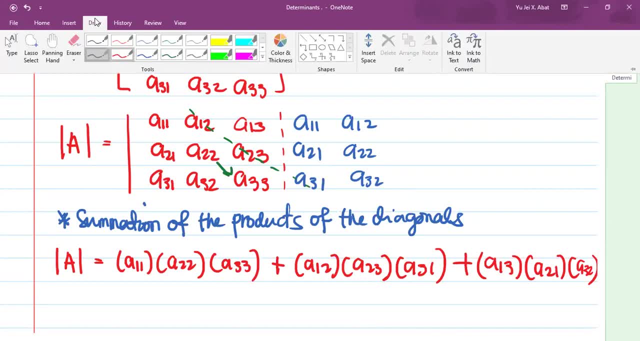 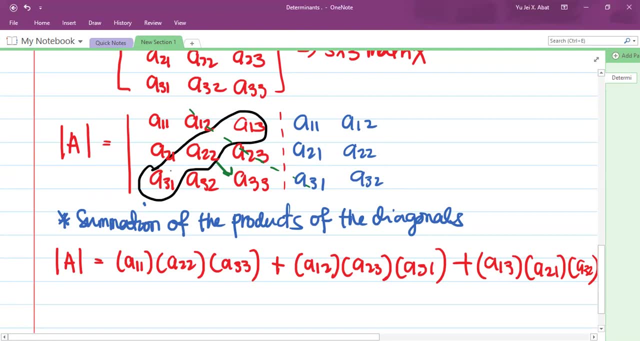 So yung other diagonal naman yung magiging target natin. So that is minus the first diagonal pataas naman. Okay? Paganyan yan. Okay? So anong mangyari dito, guys? Ito ay magiging minus. 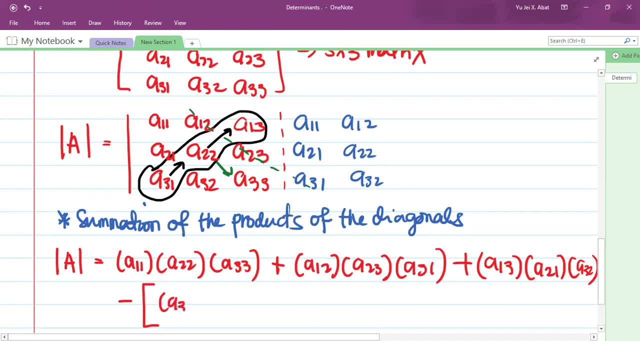 The summation of the products of A31. Laging minus. Kapag nagpalit ka na ng diagonal. Then plus pa rin kasi summation of products. 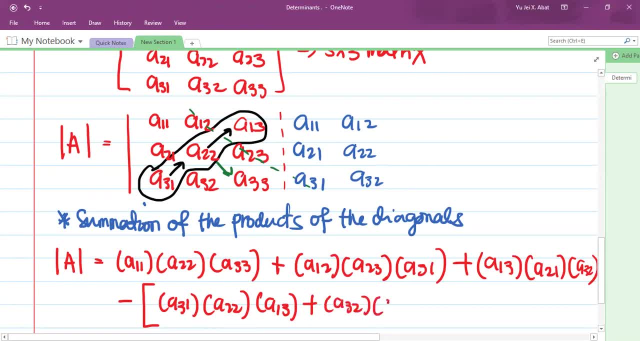 So that would be A32, A23, and then A11. Saan ang galing yun? Ito po yun. 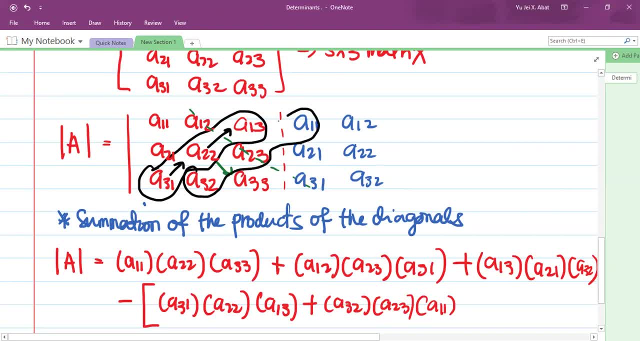 A32, A23, A11. Okay? So yan. 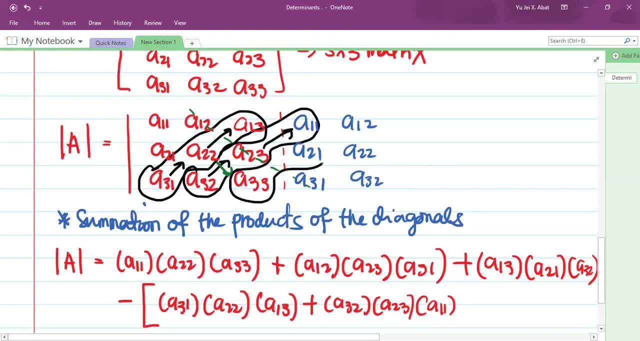 Yan yung other diagonal. Then the last diagonal would be A33, A21, and A12. That would be the last diagonal. That would be the last diagonal. 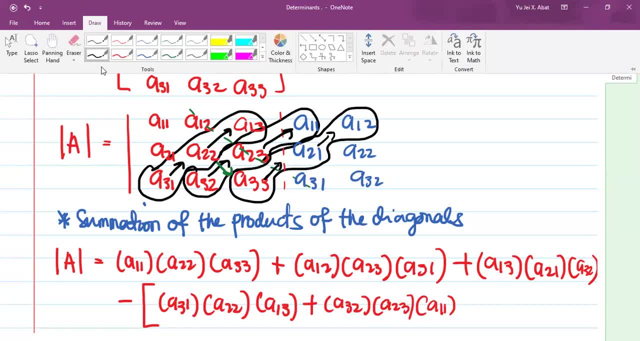 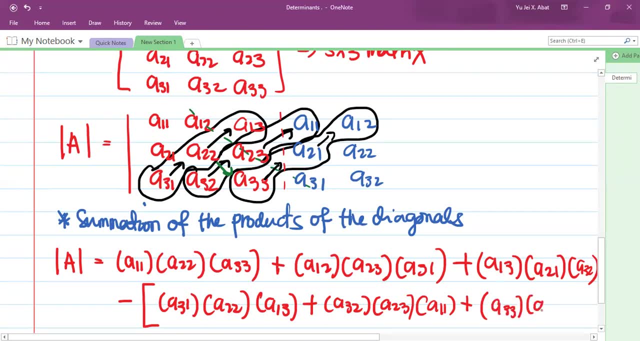 So ganun lang din. Summation of products. So plus pa rin to. Then we have A33, A21, and then A12. Ayan. So don't forget the minus. 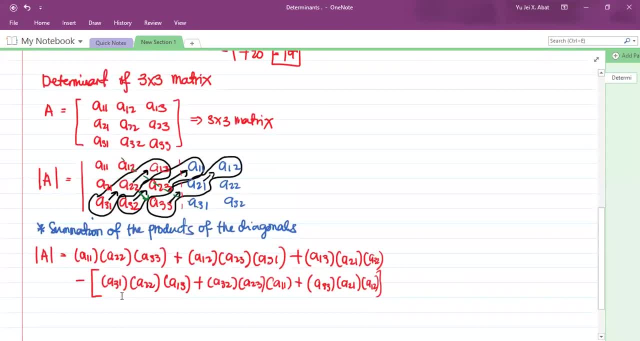 So ngayon ito yung formula niyan. Pero hindi natin kakabisaduhin kasi apakahaba ng formula na yan. 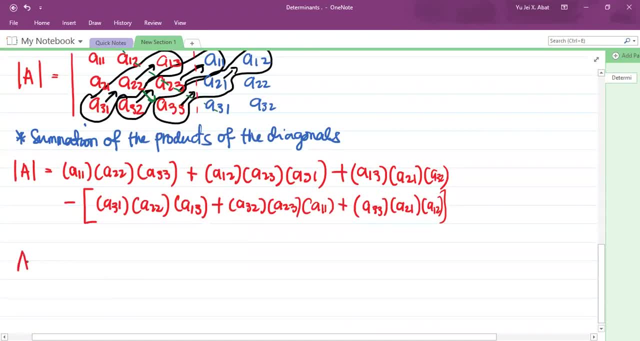 Instead, if you're going to apply it in real life, for example, we have, or in real problem I mean, 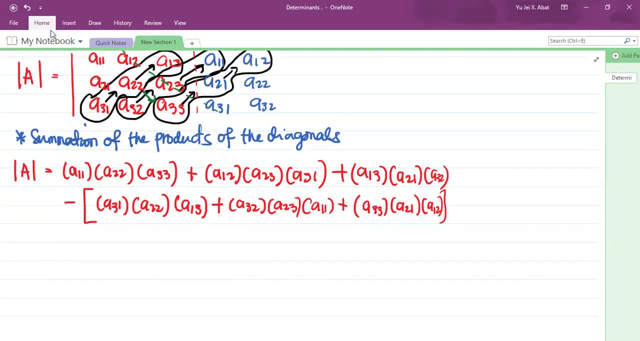 we have here, we have here, for example, matrix A. Okay? 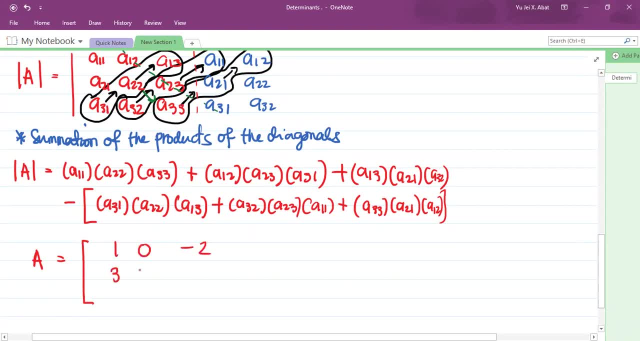 So kung meron tayong 1, 0, negative 2, 3, 1, 1, negative 1, 2, and 0, if we wish to find the determinant of matrix A, that would be what? 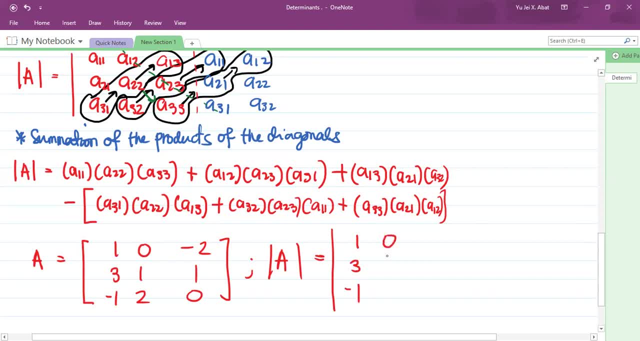 1, 3, negative 1, 0, 1, 2, negative 2, 1, 0, and kukopihin ko yung dalawang first column, 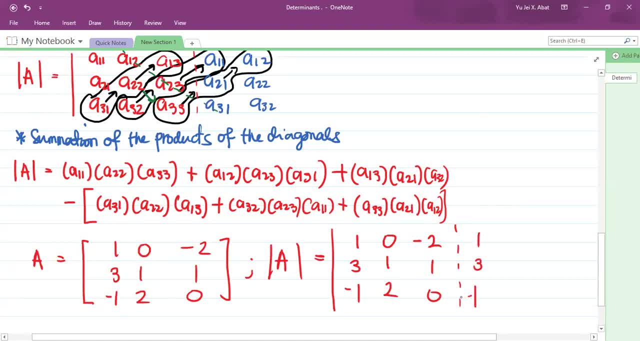 which is 1, 3, 1, or negative 1, and 0, 1, 2. So iperform natin yung determinant niya. 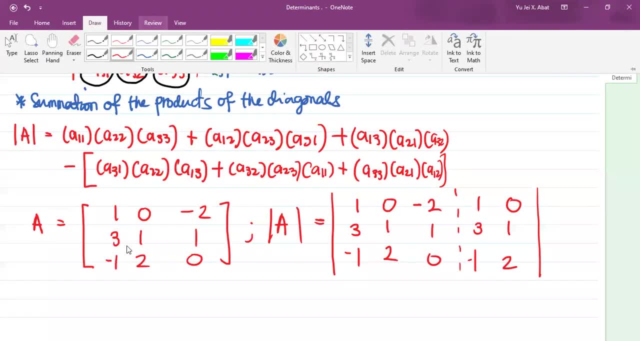 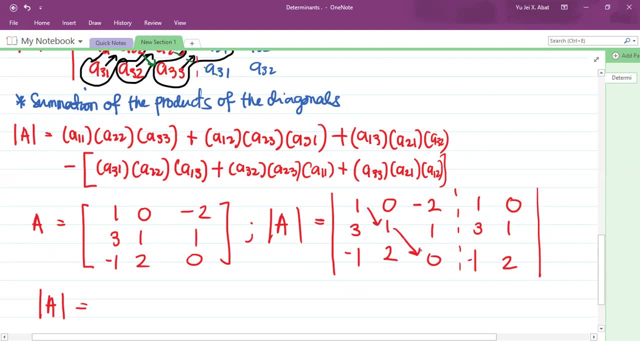 So again, performing the determinant for the matrix A, the first diagonal we encounter is this. 1 times 1 times 0. So 1 times 1 times 0 plus the other diagonal, 0 times 1 times negative 1. Swerte natin kasi meron lang tayong 0, no? And then 2 times 3 times 2. Okay. Plus? 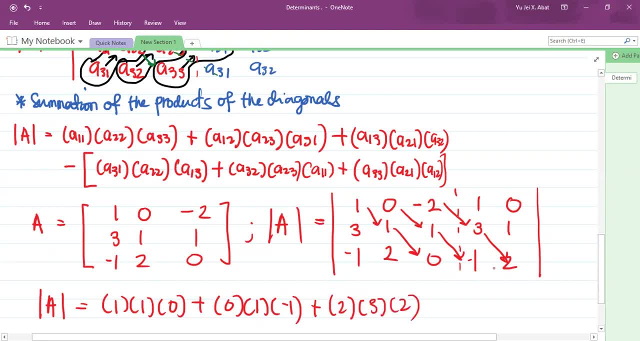 2 times 3 times 2. Okay? 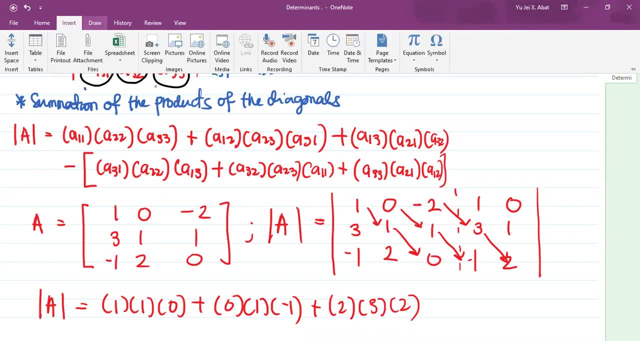 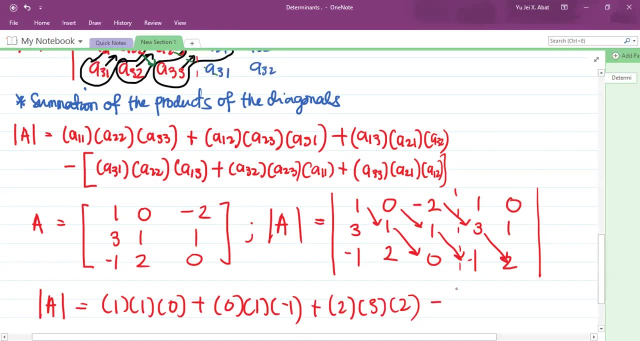 Going the other side of the diagonal, kakabilang side naman tayo, so magkakaroon tayo ng minus. So maminus natin ito. Then going to the other side, so we have negative 1 times 1 times 2. 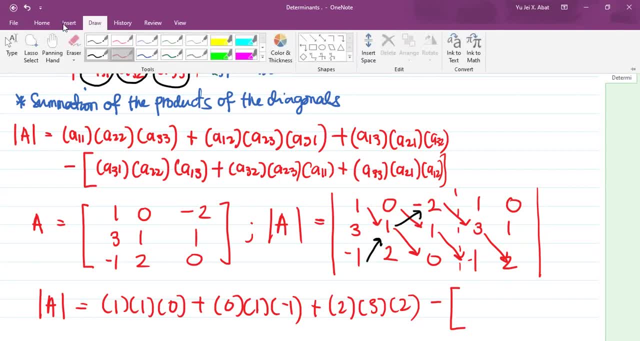 Hindi lang masyadong ayos yung pagkaka... pero diagonal yan. 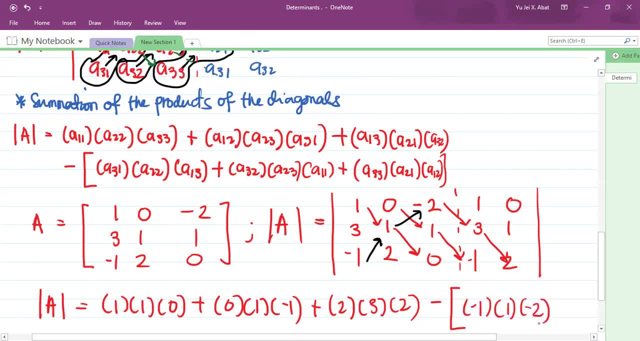 Negative 1 times 1 times negative 2. Then we have the other one. 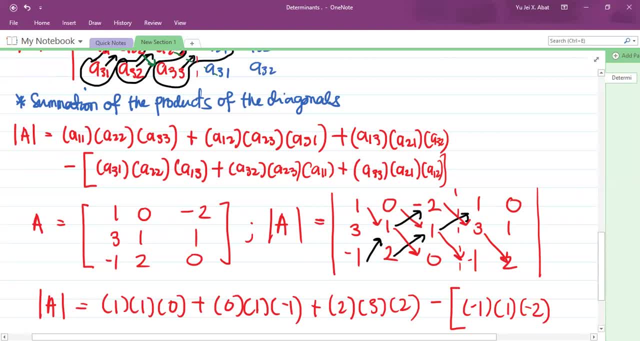 Okay, so we have 2 times 1 times 1. Okay. 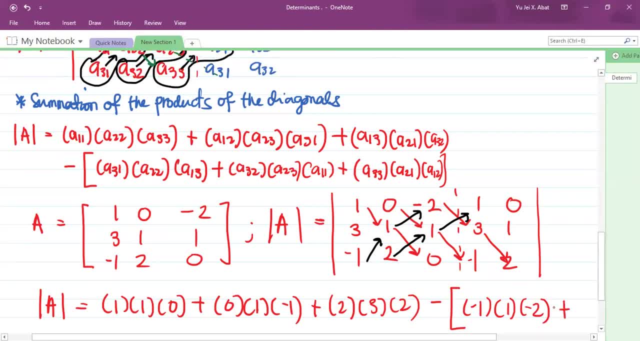 So pwedeng rektan ha, pero maganda complete solution. Again, plus yan. 2 times 1 times 1. 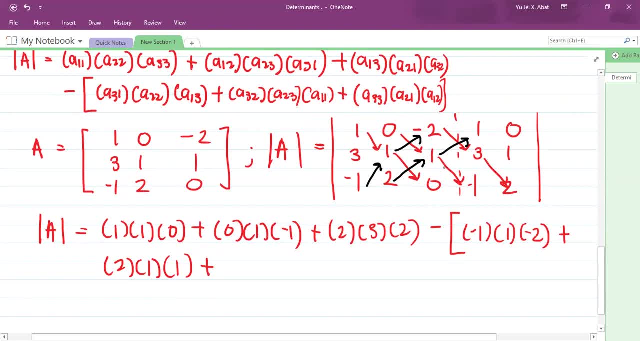 And lastly, that's plus what? 0 times 3 times 0. 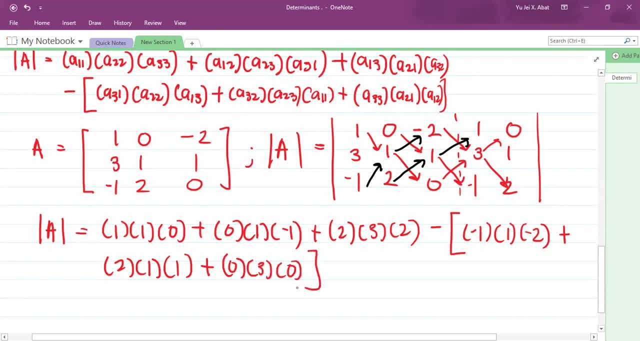 Then we have parenthesis. Okay? 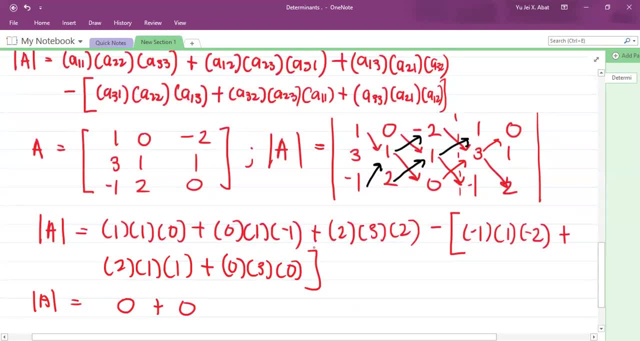 So 1 1 times 0, that's 0. And then the another one is 0. 2 times 3 is 6. Times 2 is 12. Ito yun. Then minus. 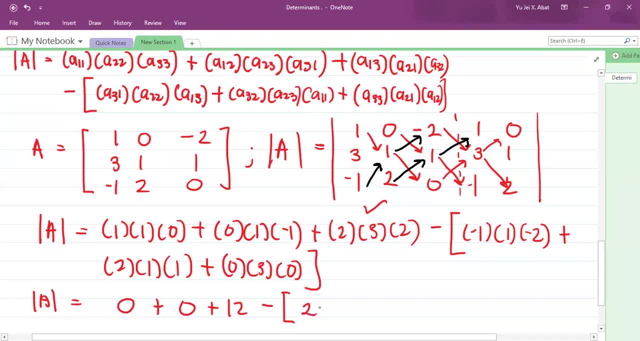 Okay. Negative 1 times negative 2 is 2. Times 1 is 2. Plus 2. And then plus 0. Okay. So you have there 12. Okay. And then we have 4. 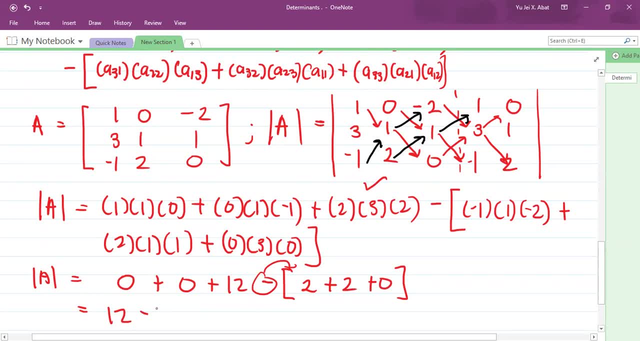 So may minus sign ka dito. Distribute mo. 2 plus 2 is 4. So minus 4, that is 8. That is our determinant. 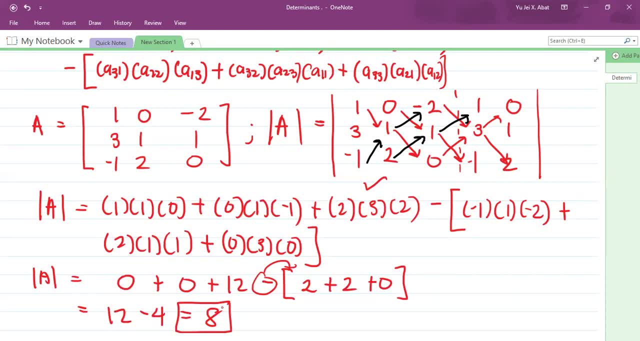 Question, guys. Wala pa naman, sir. 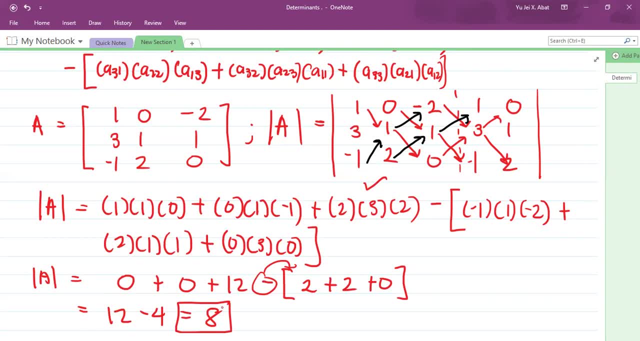 Clear naman, clear. Clear na, clear pa. Wala pa, sir. 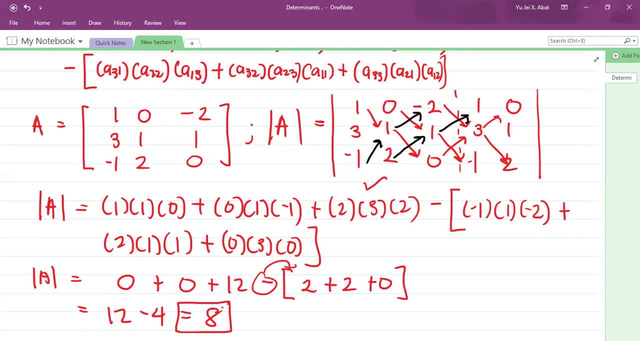 So ganoon maghanap ng 3 by 3. So iba't-ibang technique sila. Yung 2 by 2, it's the easiest. 3 by 3, kailangan lang kopyahin yung first 2 columns. And then follow the basket type, I think. Yun ang tawag nila dito. 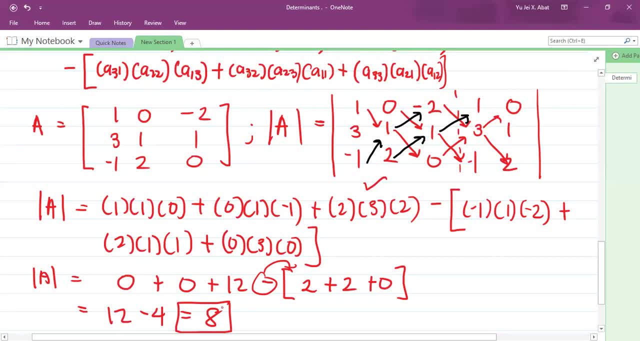 Basket type of method of getting the determinant. By copying the first 2 columns. So yun yun. 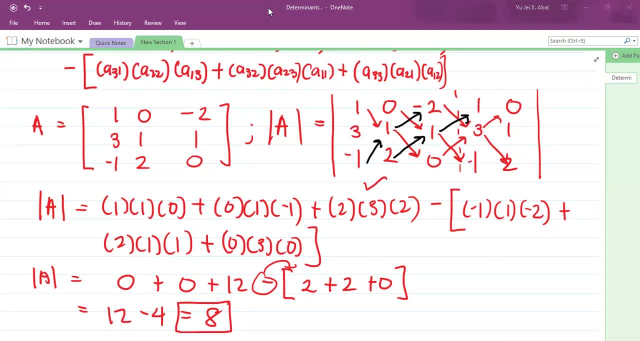 Okay. So I just want to follow the first 2 columns. 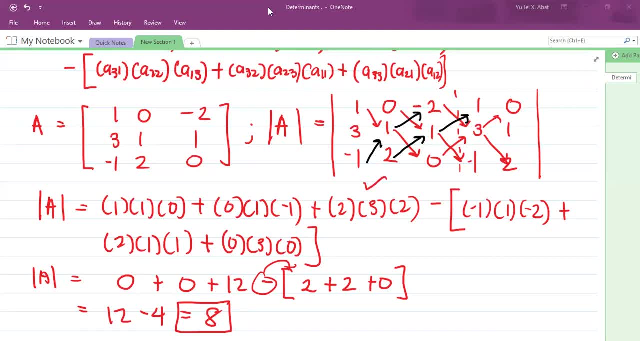 It was no spontaneous." I think that's the word I used. But here, you will also run through the년 Hello. Wait lang guys. Wait lang. Saglyf. You You 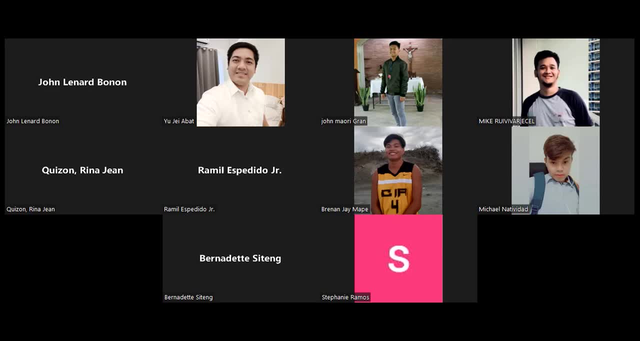 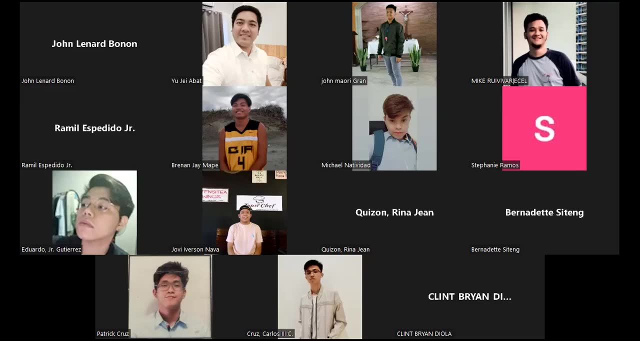 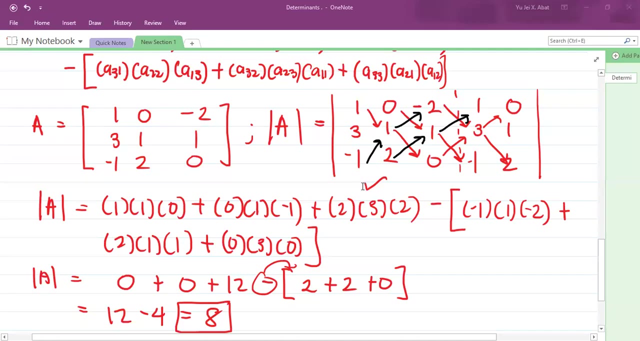 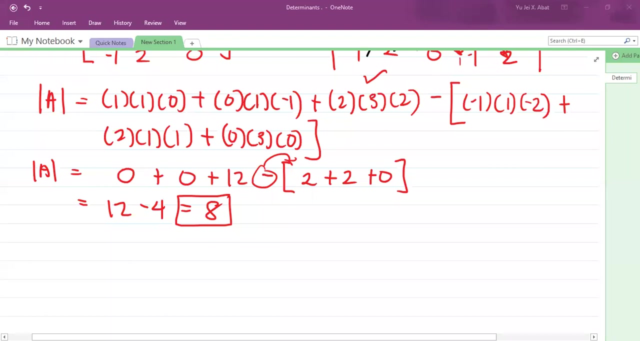 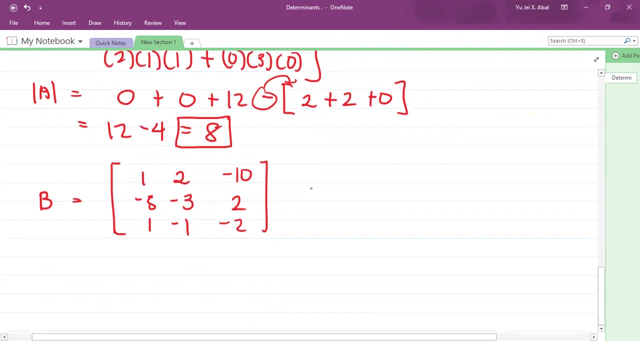 All right, so thank you so much for reading guys so far. No questions. No, I know questions. So let's try another one Let's try another one. So for example matrix B matrix B So you have A matrix B pala dapat walang absolute no sign So basta declared lang as B Kasi pag may absolute di pa si B, kinukuha na natin yung determinant So 1, 2, negative 10, negative 5, negative 3, 2, 1, negative 1, negative 2 So in order to get again the 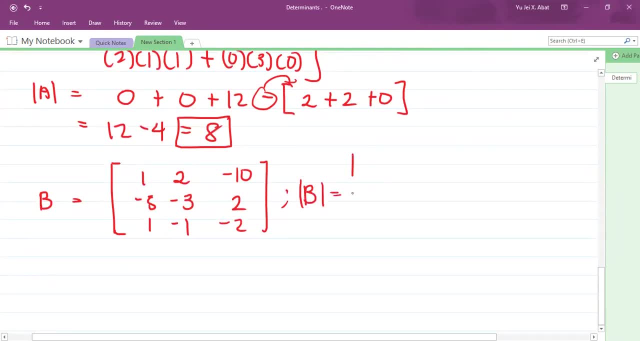 determinant of that So we should be able to copy 1, negative 5, 1 2, negative 3, negative 1 Negative 10, 2, negative 2 And copy the first two columns again So we have 1, negative 5, and 1 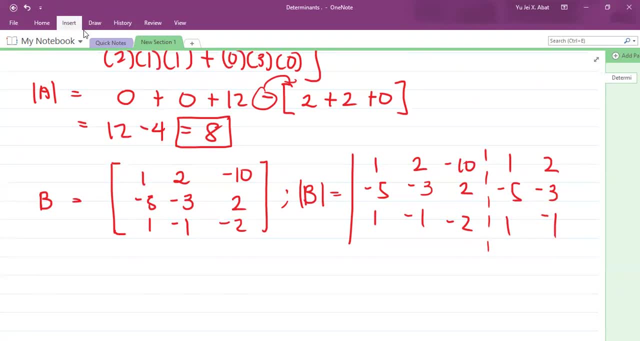 2, negative 3, and negative 1 Pag in-open natin yan 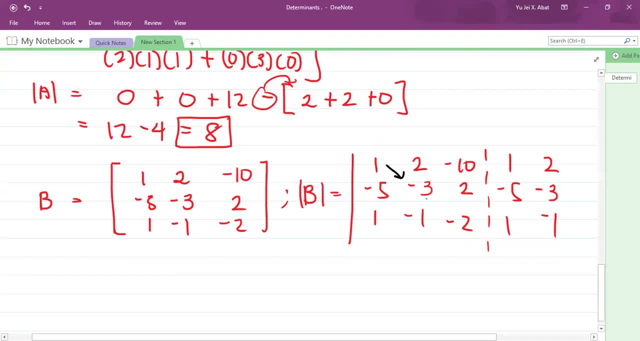 Okay, so you have this this this and this 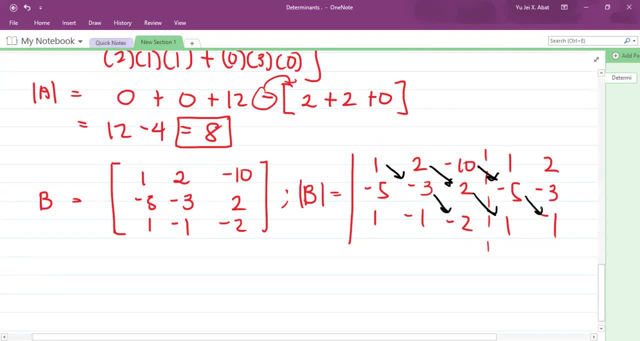 this and this one for the first diagonal Okay, so let's say the determinant of B that would be 1 times negative 3 times negative 2 plus 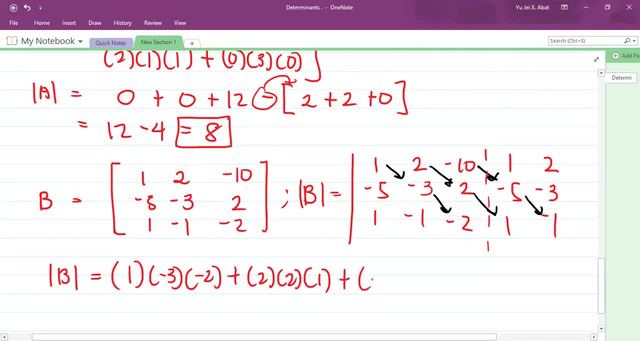 We have 2 times 2 times 1 Plus we have negative 10 times negative 5 times negative 1 Then minus minus So minus we have 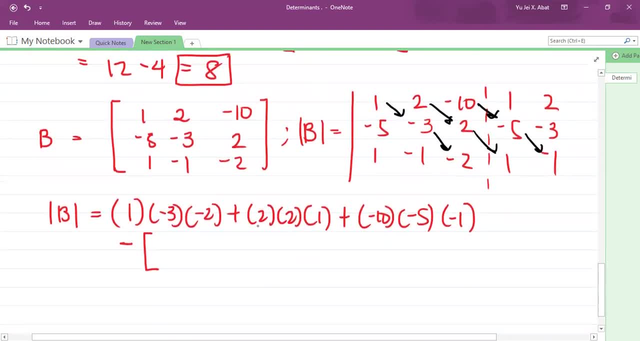 ah ah We have yung other diagonal This one This one Ayan 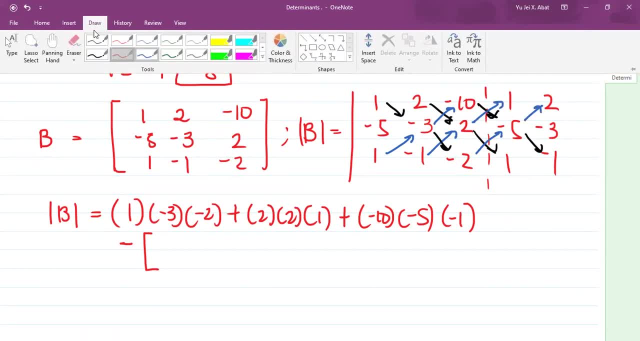 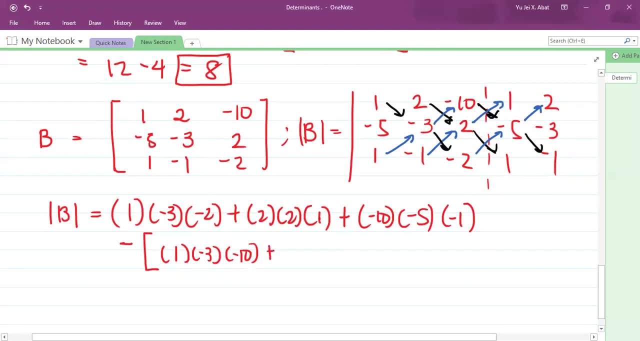 So yan na yung magiging diagonals natin guys So minus don't forget na minus na So you have 1 times negative 3 times negative 10 Plus pa rin Since summation ng products pero other diagonal na to Negative 1 times 2 times 1 Plus negative 2 times negative 5 times 2. So as easy as that. And then we do the arithmetic. 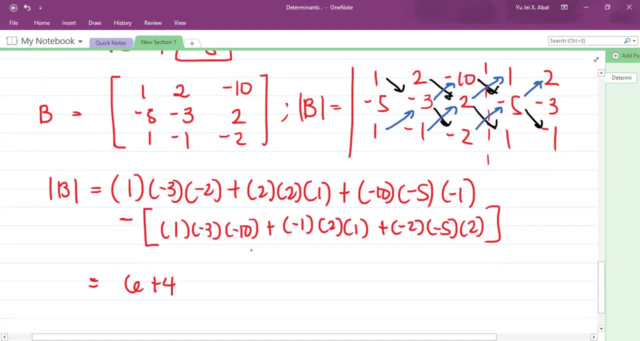 So 1 times negative 3 times negative 2, that's 6. Plus 4, that's negative 50. Positive 50 times negative 1, it's negative 50. Because there are 3 negatives. 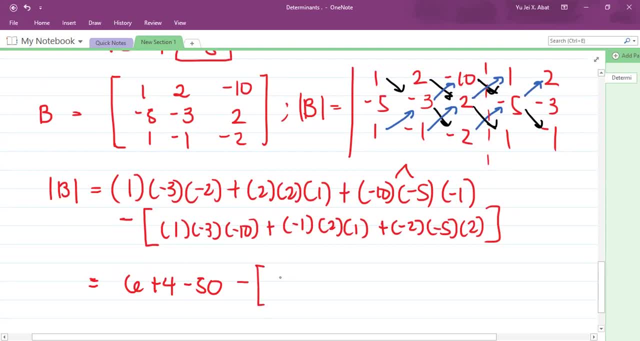 Minus, we have 30. 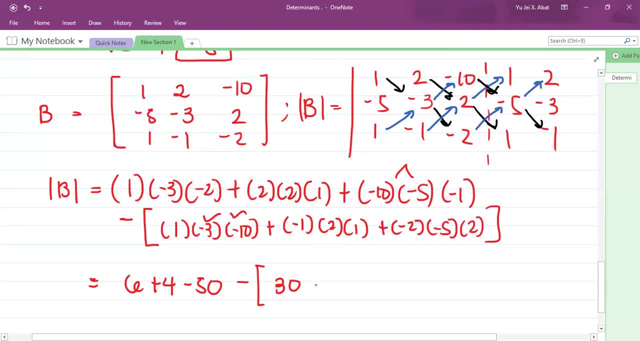 Negative 3 times negative 10. And then we have minus 2. Negative 2 times negative 5 is positive 10 times 2, 20. So let's see. 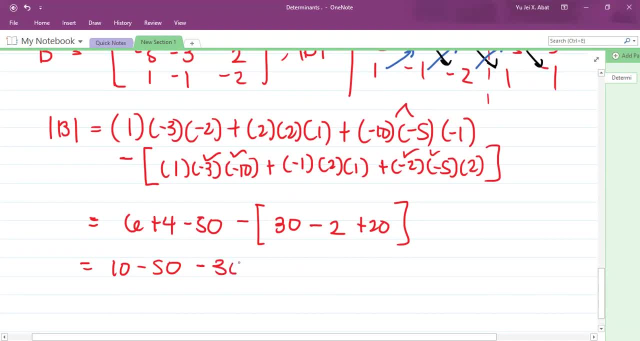 10 minus 50 minus 30 plus 2 minus 20. Or you can also... 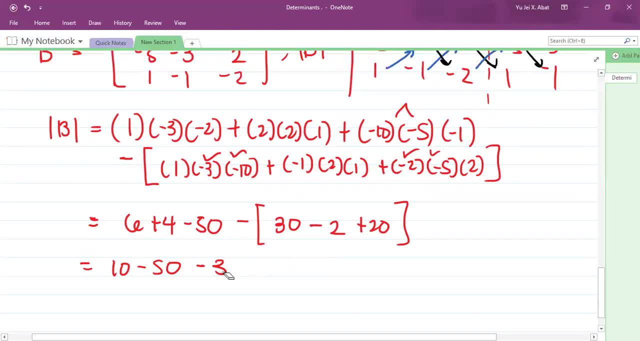 You can also simplify it first. Same thing. 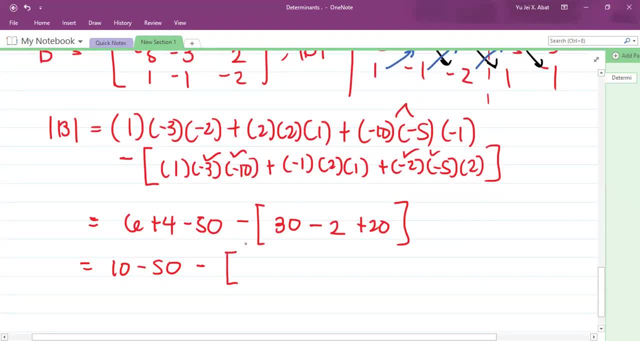 So you have 30 minus 2, it's 28. Plus 20, 48. So you have negative 40, 10 minus 50, negative 40, minus 48, that's negative 88. Correct, guys? Yes. 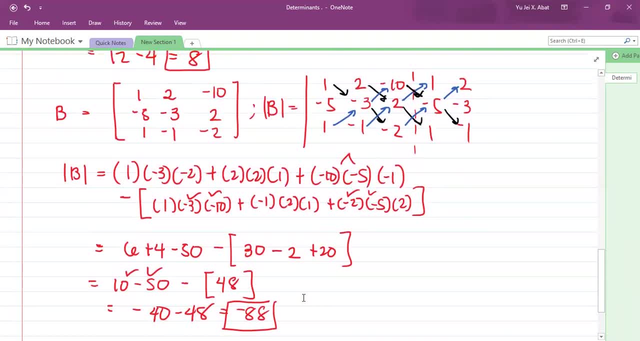 Did you understand my questions? Questions ba? Yes, sir. 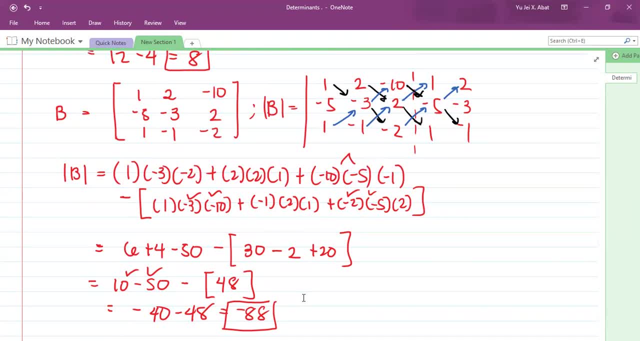 Ma'am, sir. Nakakasunod naman. Yes, sir. So that's how determinants work, no? Ayan. 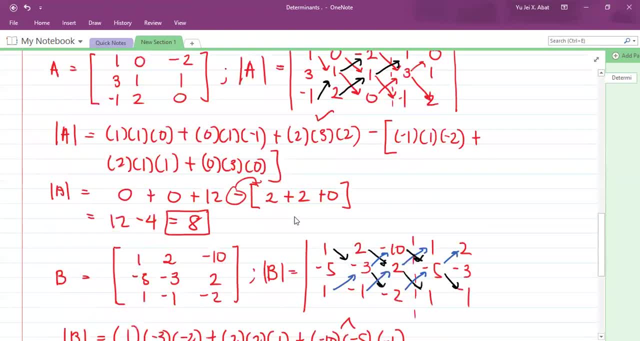 So how about for a 4x4? So 4x4 determinant. 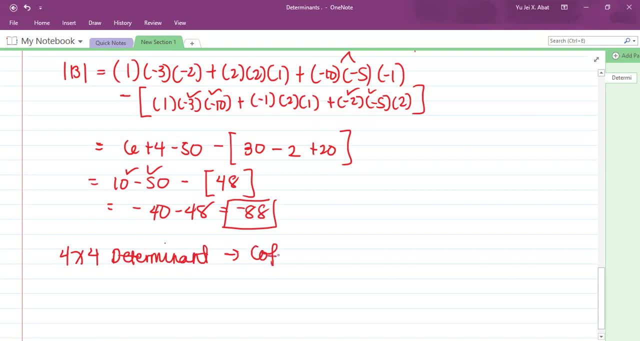 A 4x4 determinant, we are going to employ cofactor method. Okay? Pag-ibusin mo ng cofactor is we will either... 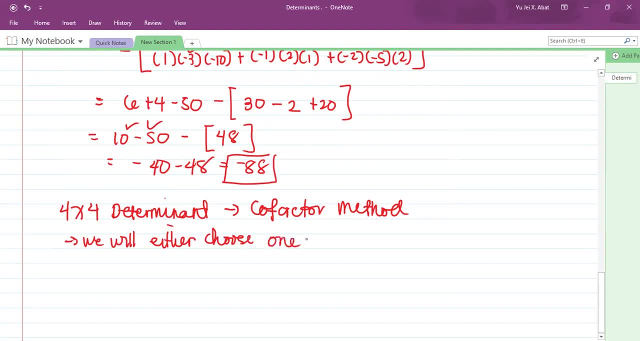 choose one column or one row, depende, pipili tayo, to be the cofactor. 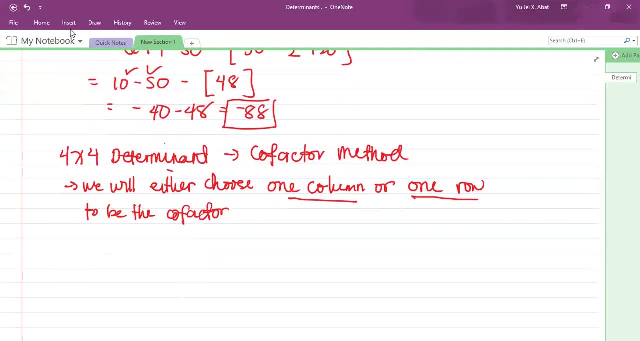 Now, meron din tayong sinusunod na sign convention. Abayin ko na lang kulay. Okay? Okay. For 4x4. 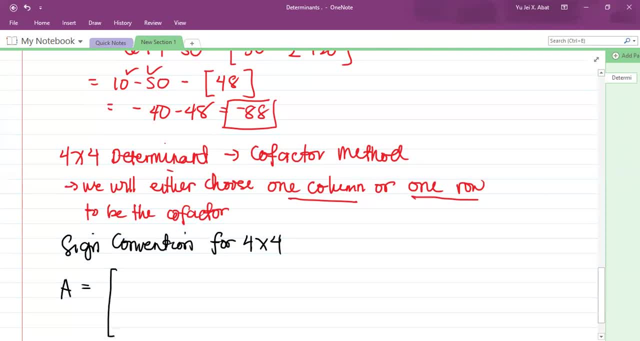 Suppose meron tayong 4x4 na matrix. Aba ko lang. 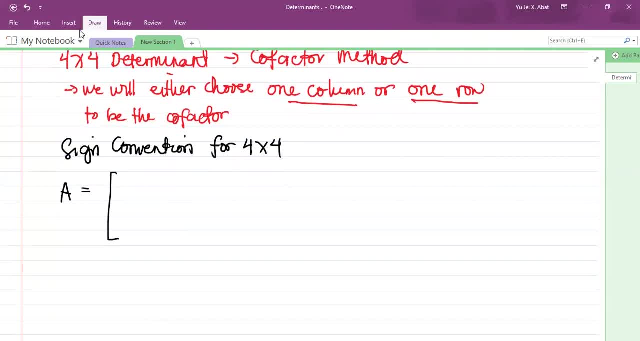 Suppose meron tayong 4x4 na matrix. Abayin ko lang, medyo maliit ito kasi. Ayan. 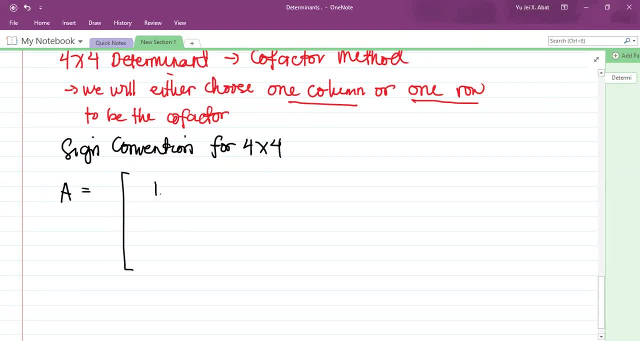 So you have... Let's say 1, 0, 8, 9, 10, 11, 12. 1, 0, 9, 10, 11, 12. 0, negative 1, 0, negative 2, 2, 0, 1, 3, 2, negative 1, 4, and then we have 6, 2, negative 1, and 2. 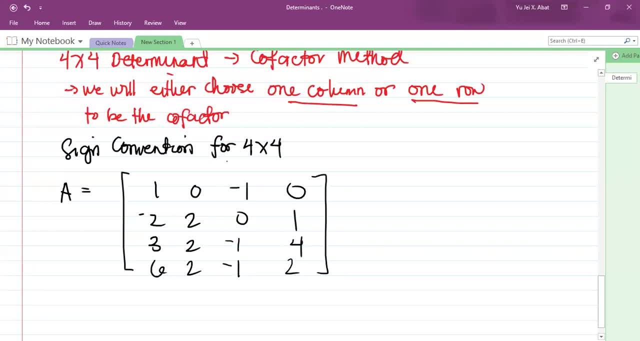 For example, 4 by 4, 4 rows, 4 columns. Magiging sign convention yan is kapag gumamit tayo ng cofactor method is ganito. 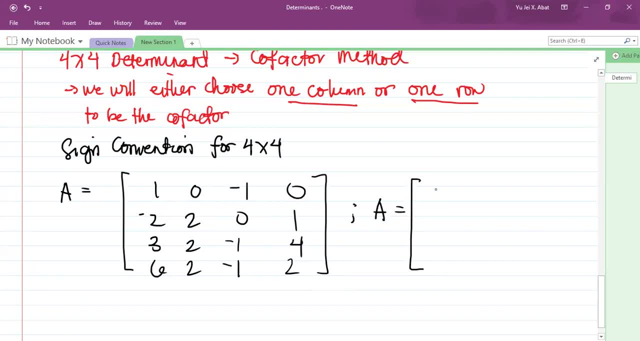 Ibig sabihin ng sign convention, yan yung susundin natin. Positive, negative, positive, negative. 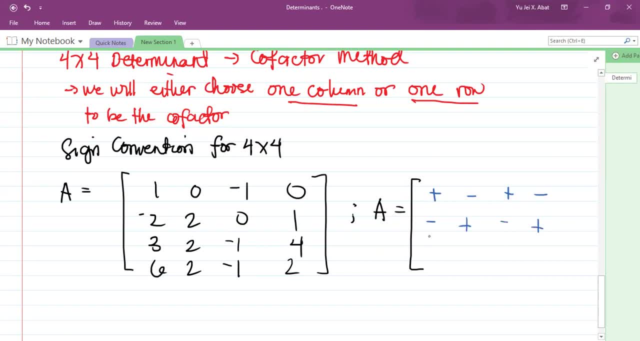 Negative, positive, negative, positive. Positive, negative, positive, negative, negative, positive. So then positive, negative. 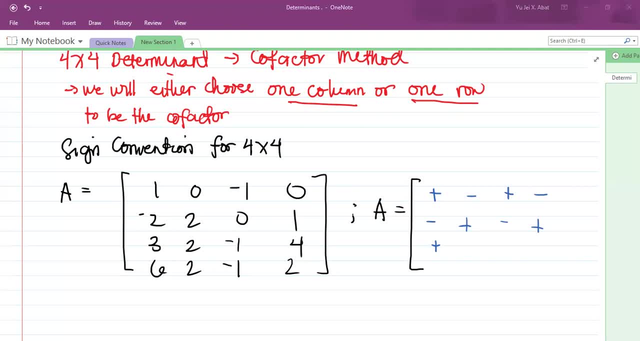 Wait lang. May naka-pop up sa aking screen at ang ingay. Yan. 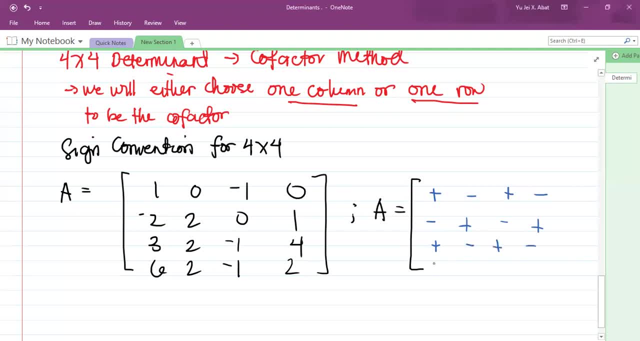 Then positive, negative, positive, negative. Then negative, positive, negative, positive. 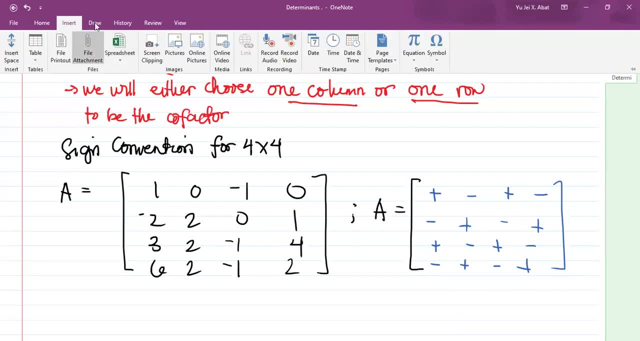 So basically, meron tayong sign convention and this is our sign convention. Ayusin ko lang. 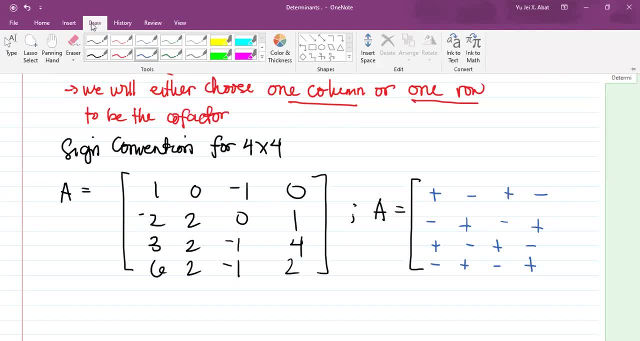 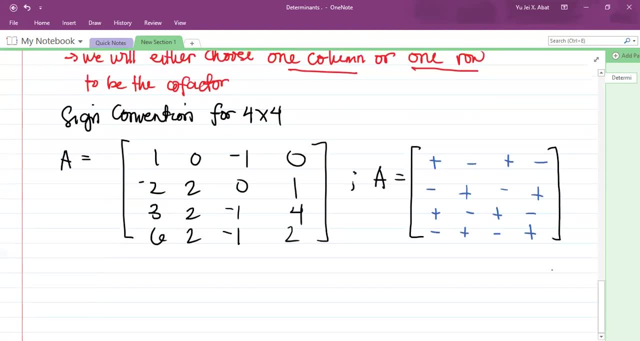 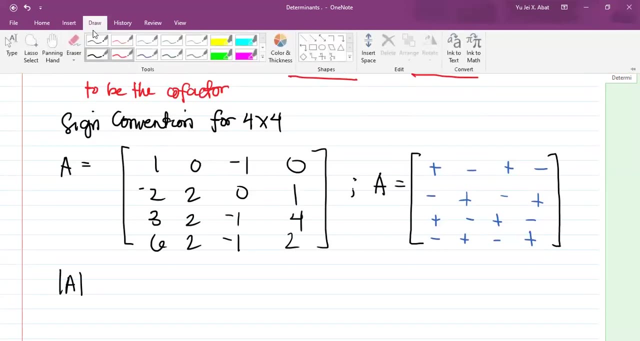 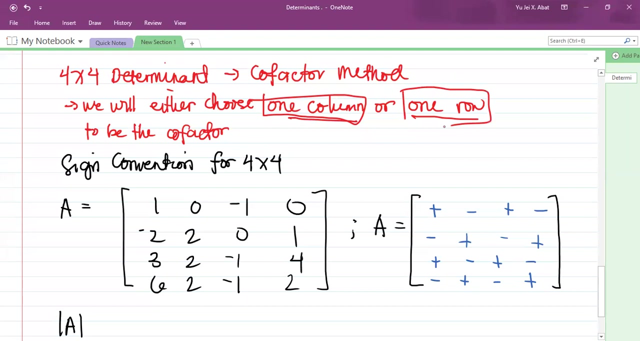 So paano ba yun, sir? For example, gusto mong kunin yung determinant ng A. Either, ang sabi ng instruction natin, pipili ka ng isang column or pipili ka ng isang row. Kasi i-e-extract mo yan. For example, Okay, for example, 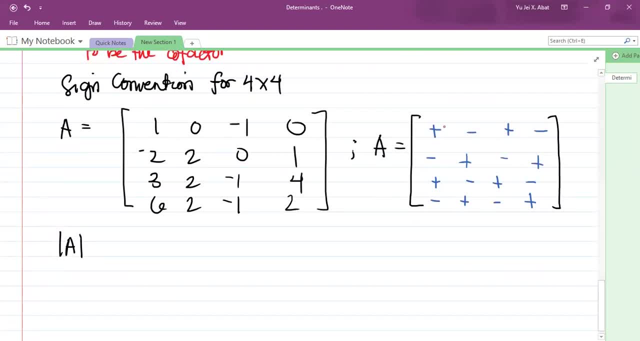 Pumili ka ng isang row or isang column. Pwede natin piliin yung maraming zero kasi mas mapapadali yung solution natin dyan. So let's say, pinili ko to. Ayan. 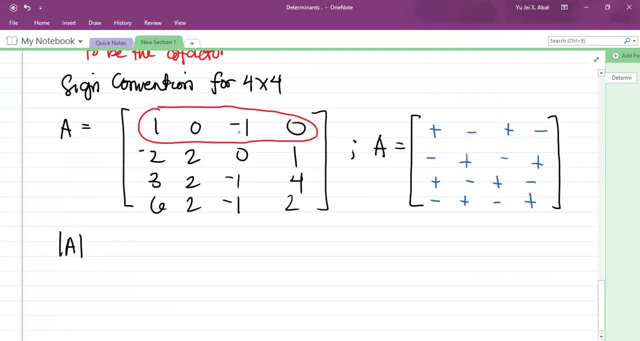 Okay. So kung pinili ko yan kasi may zero, yan yung row one. Okay. 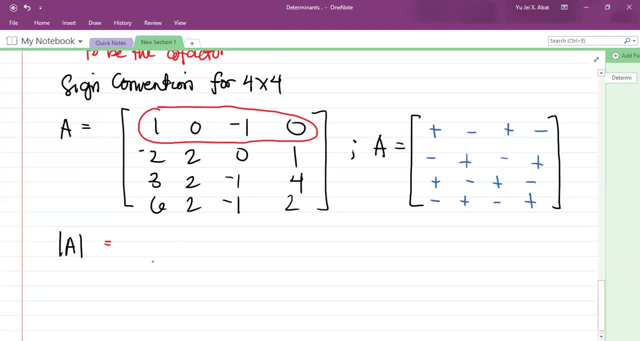 So from there, kukunin ko yung mga constant nyan. So magiging one, then may determinant ako. Okay. Okay. 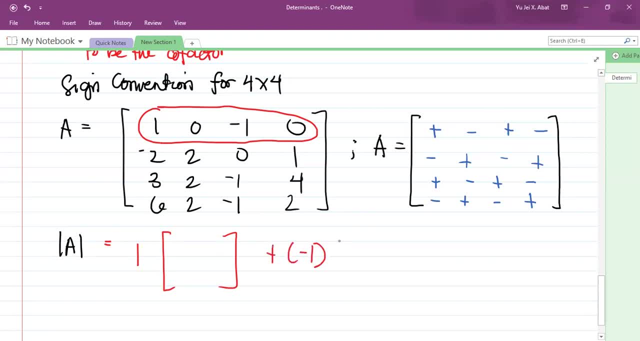 Then meron akong... plus negative one, okay, dahil may determinant ako, and then so on and so forth. So parang ganito yung mangyayari. 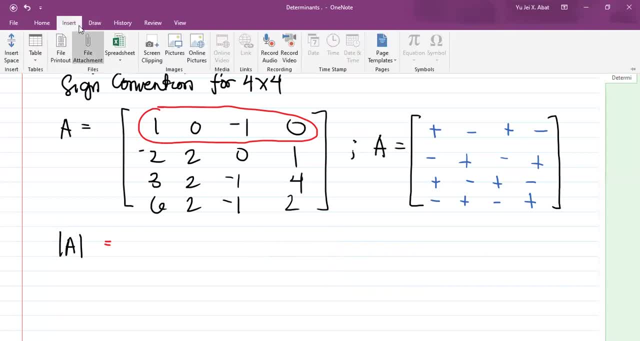 Okay. Pag kinuha ko yan, yung buong row na yan, so ganito. Okay. Okay. 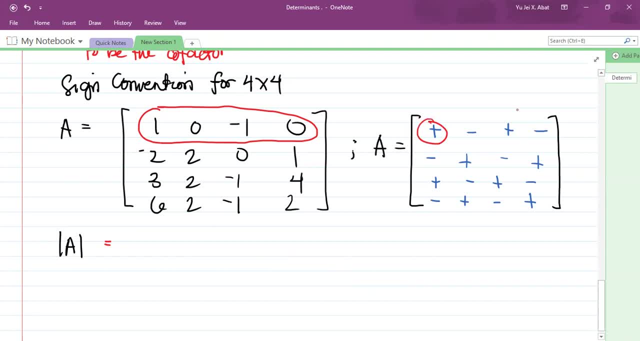 Applying the sign convention, sabi nung... Dahil ito yung gagamitin kong sign convention. Okay. So kung baga, yan yung magagamit kong sign convention. 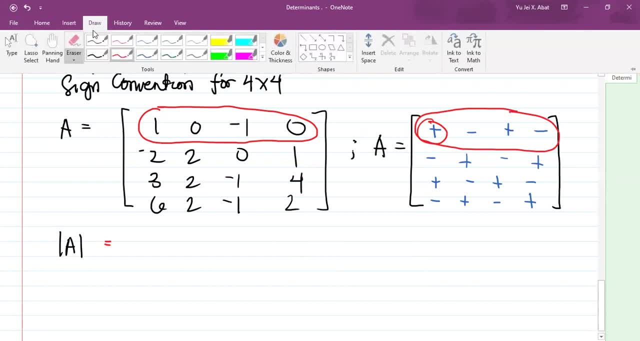 So now, pinili ko yung una. So magkakaroon ako ng one. 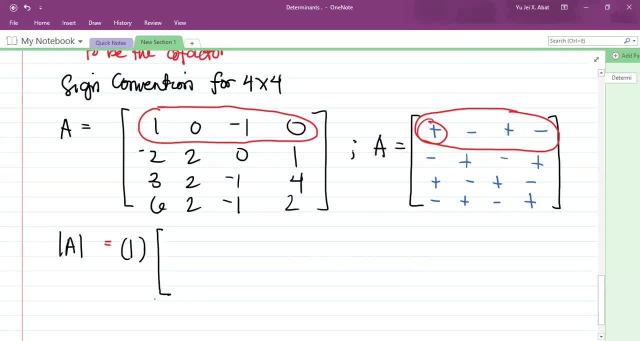 One times, okay, the determinant ng may iwan. 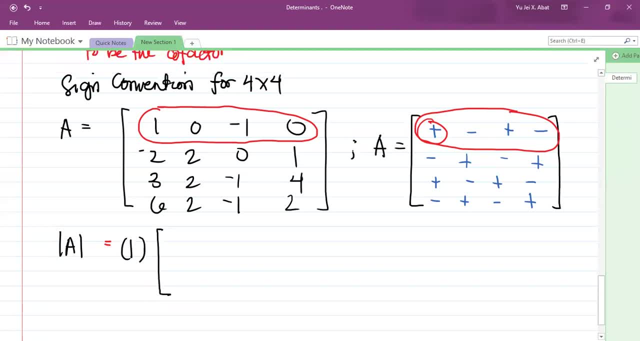 So kung ito yung aking piniling four factor, okay, yung buong ito ay canceled, at yung buong row na ito, canceled. Ano yung naiwan na matrix? Ito. So yan ang isusulat ko. So magiging... 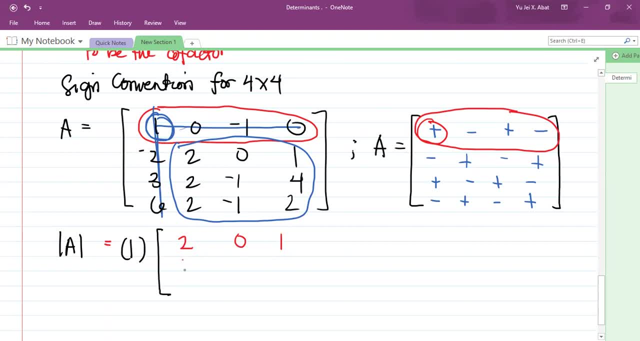 two, zero, one, two, negative one, four, two, negative one, two. Applying the sign convention na positive yung one ko. Okay. 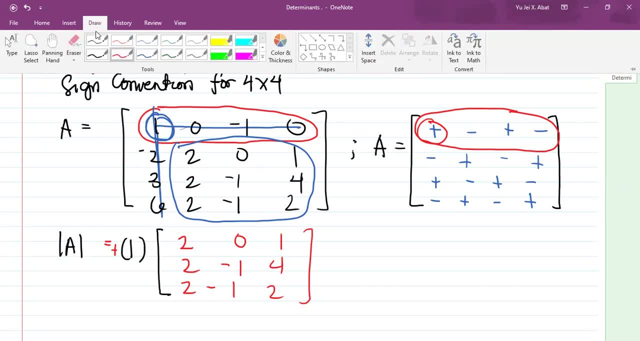 Then, nagets ba yung part na yun, guys? Nagets yun? Okay. 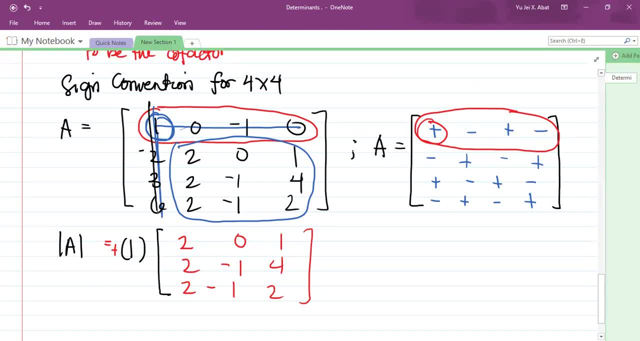 So I'm going to cross out this column and this row. Okay? 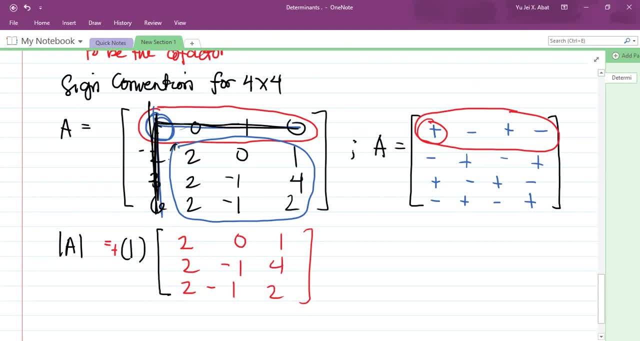 And then, kukunin ko yung natirang matrix, which is ito yun. Nagets nyo? Kuha? Yes, sir. 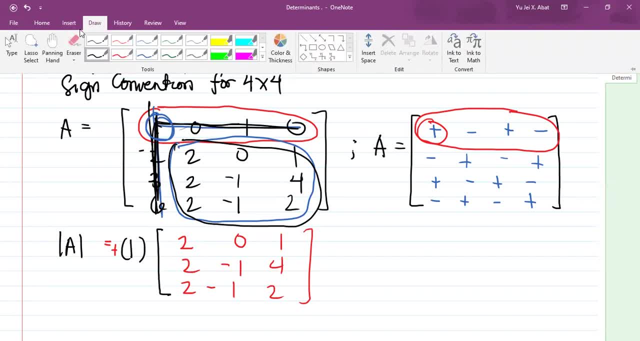 Okay. So ngayon, magigets nyo na yung pangalawa. Magigets nyo na yan. So tanggalin ko lang yung mga pinagagawa ko. Okay. Borahin ko lang. Ulit. Pero yan pa rin yung cofactor natin. Okay. Yung row na yan. Row one. 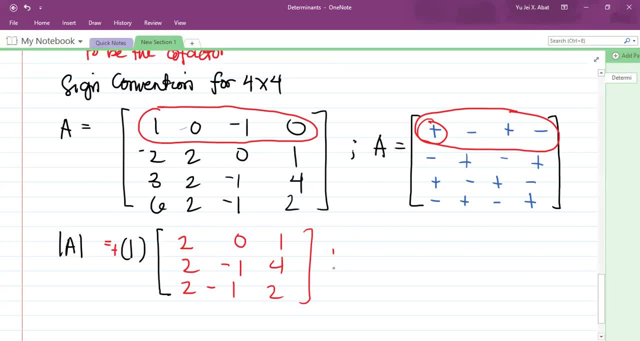 So yung pangalawa naman, guys. Para di ka malito, add mo lang yung plus. Basta plus lang. Okay? Laging ganyan. Plus. Eh may negative na dito. So ito yun. Yung zero. 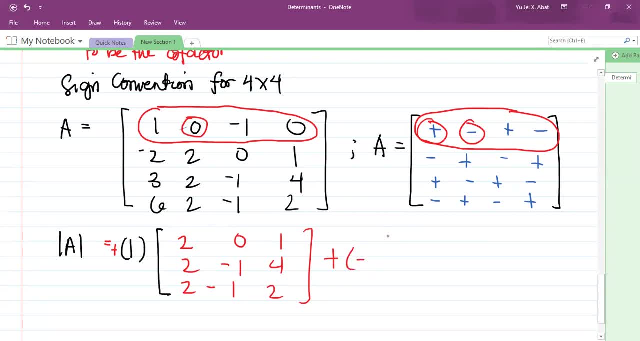 So meron kang negative ng value na yun. Okay? Or pwedeng rekta negative. Okay? So negative of zero. So kasi naman, 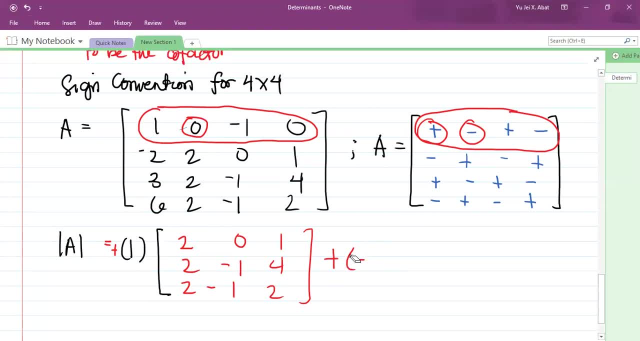 pag positive naman ilagay mo dyan, negative of positive, magiging negative. So pwede mo na rin ilagay na minus. Diba? 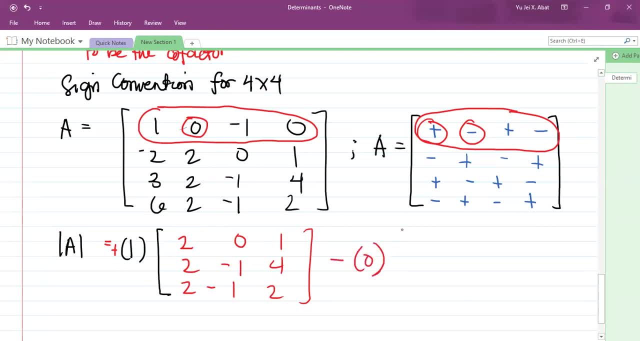 So magiging minus zero times. Ayan. 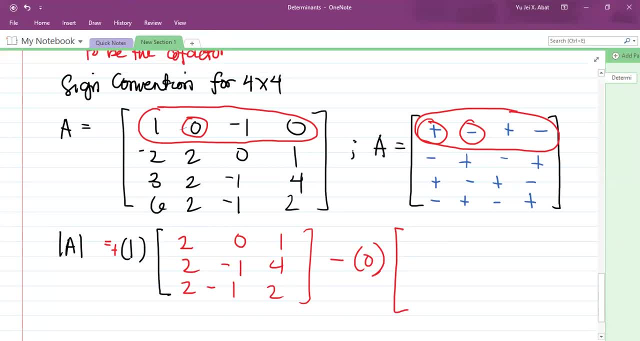 So ang susunod mo naman gagawin is you're going to cover yung 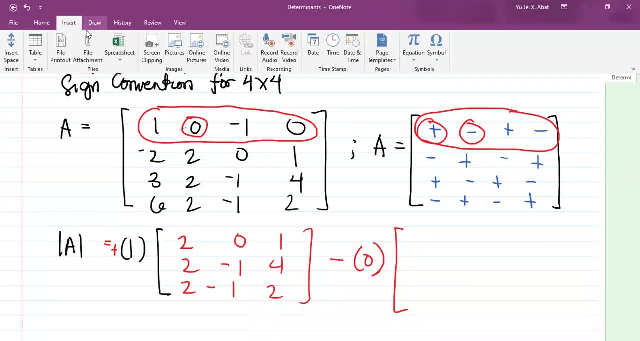 column ni zero. Yung column na kung anong pinabibilangan niya. 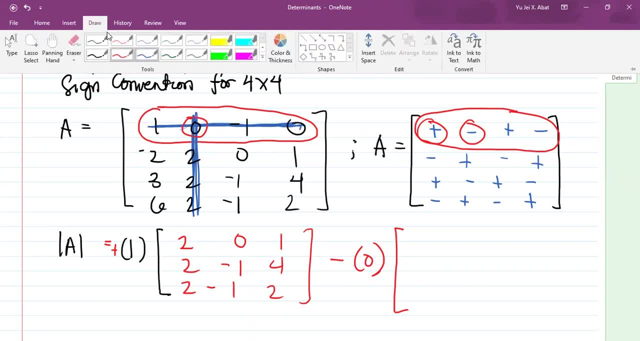 So anong natira guys? Merong matitira na matrix. 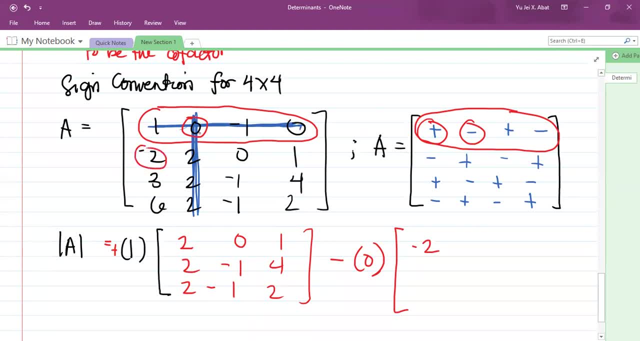 So ano yun? That's negative two, zero, one. You have three, negative one, and four. Three, negative one, and four. And then six, negative two. Negative one, and two. 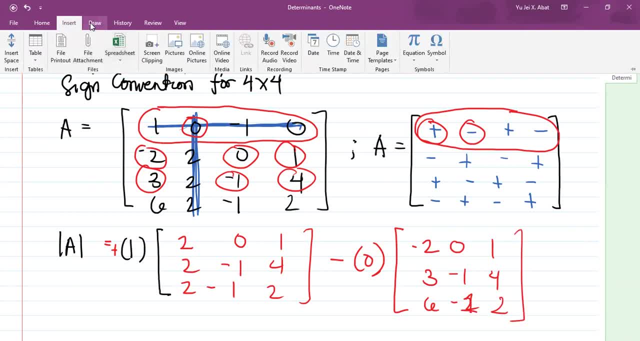 What's good about it is kahit makuha mo yung determination, kahit makuha mo yung determinant nito, kahit kasi determinant to eh. 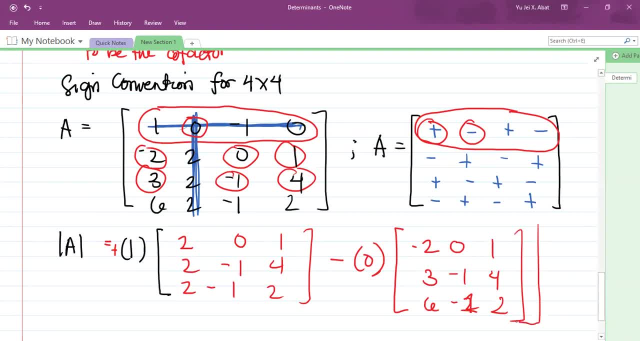 Determinant to. Eto. Determinant yan. So kahit makuha may determinant yan, 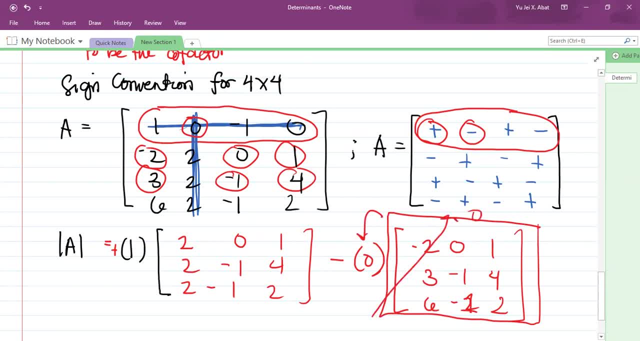 imumultiply mo sa zero, eh di zero na yung whole na ano yan. Diba? 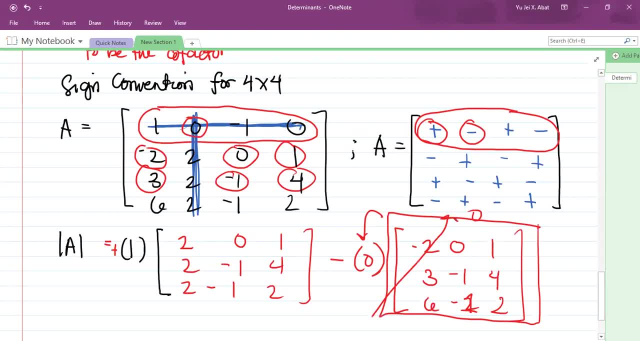 Kaya nga yung ina-advise ko, yung may rows na may zero or columns na may zero, maganda yun. 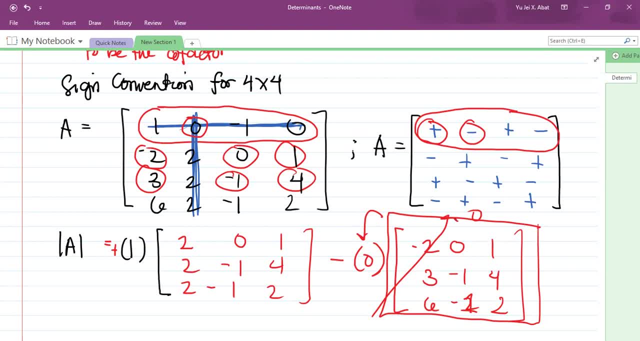 Kunin as co-factor. Though kahit ano naman dyan, kahit anong row, kahit anong column pwede. Okay? So yan. For the purpose lang na gano'n. 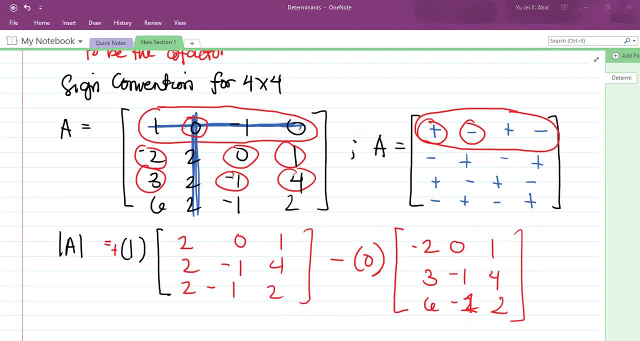 Ang daming chat, wait lang. Wala ko bakit ba lumalabas na dito. Isa na tayo. Ayan. So nag-gets na yung part na yun. Okay? Nag-gets ba? Guys? Nag-gets. 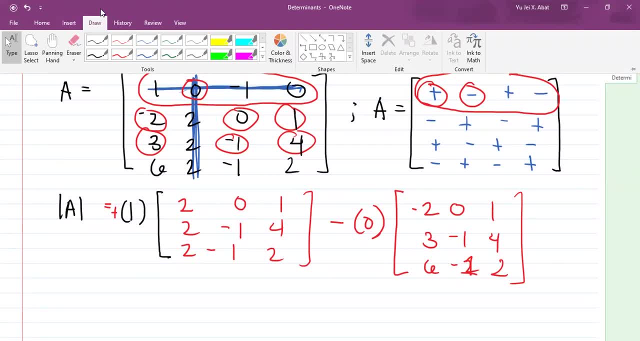 So ngayon, nandun na tayo sa pangatlong co-factor. Okay. Moving on na tayo. 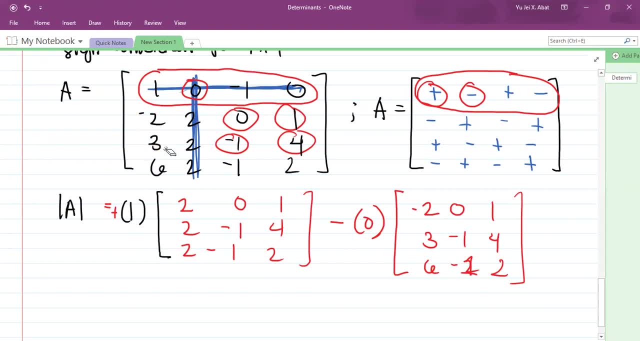 So gurahin ko lang ulit yung mga in-encircle ko dito. 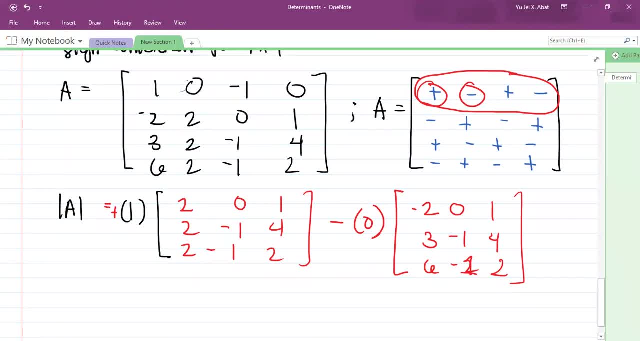 Diba? Zero yun. Nag-lagay ko dyan. Nabura rin na yan. So again, yung co-factor natin, pinili ko to. So nasa na tayo? Nasa negative one na tayo. So anong mangyayari? Okay? Okay? 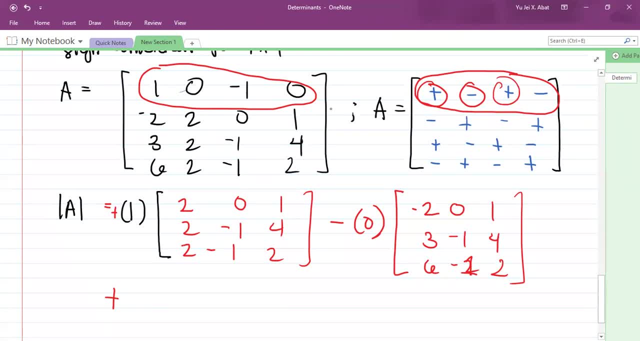 So dahil negative one to at plus convention to. Okay? Plus ka lang din. 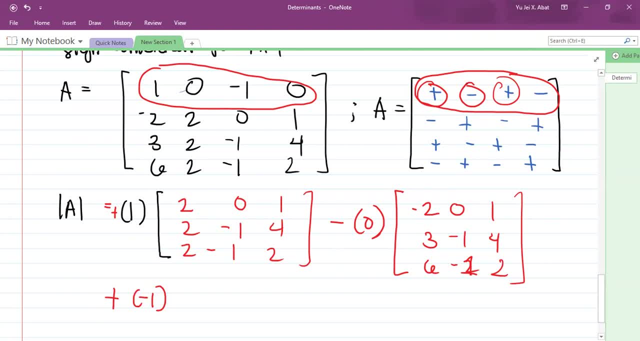 Negative one. Plus kasi nga positive na to. 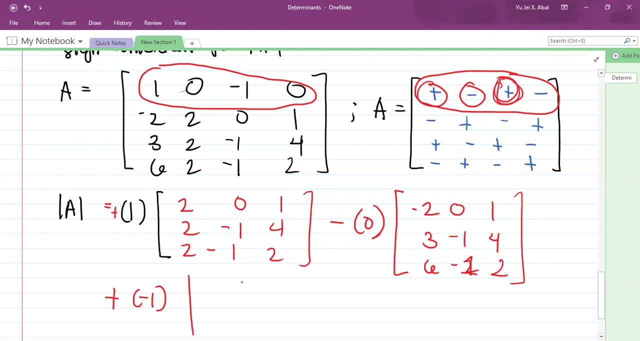 Kaya plus. And then yung determinant naman nung matitira. So pag pinili ko naman to guys, ang maka-cover nya ito at ito. Laging yung row one. Okay? 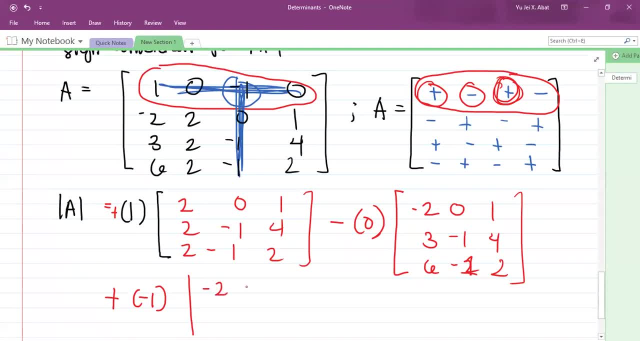 So anong makapili nya? Meron kang negative two, two and one. Three, two and four. 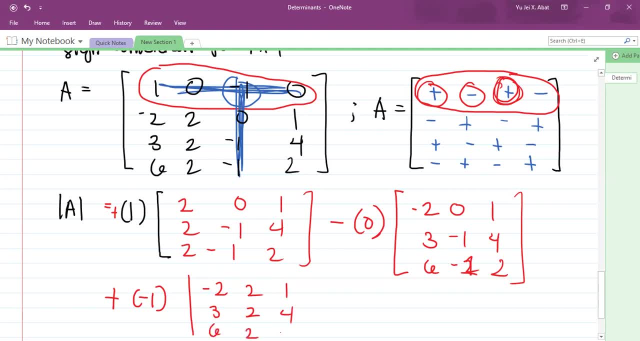 Meron ka rin six, two and two. Determinant yan ah. So sorry palitan natin to determinant. Dapat yung hindi sya matrix. Determinant sya. So determinant ibig sabihin absolute. 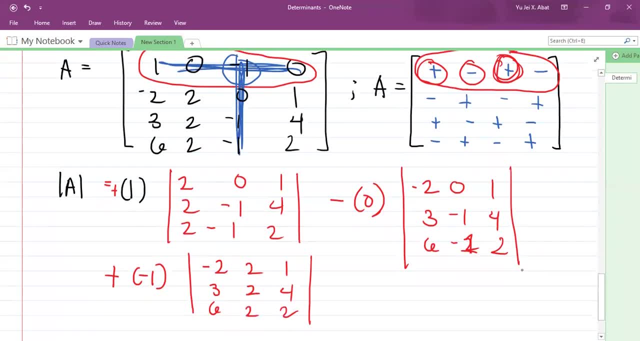 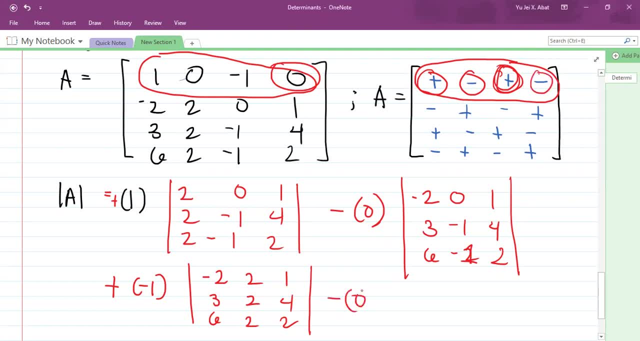 So minus. Dito. Minus zero times kung ano yung matatakpan niya. May iwanan niya. Ano ba yun? So, itong row yun, takip to. Takip din to. 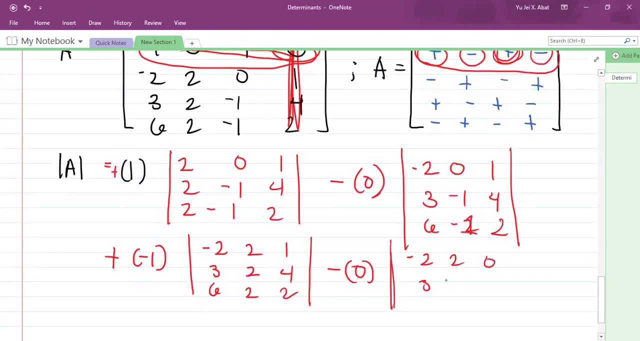 So, negative two, two zero, three two negative one, six two negative one. Ayan. 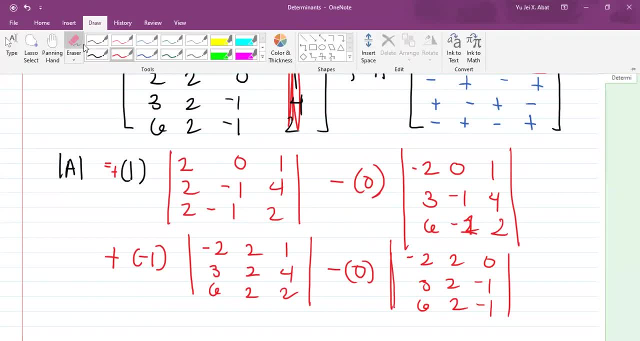 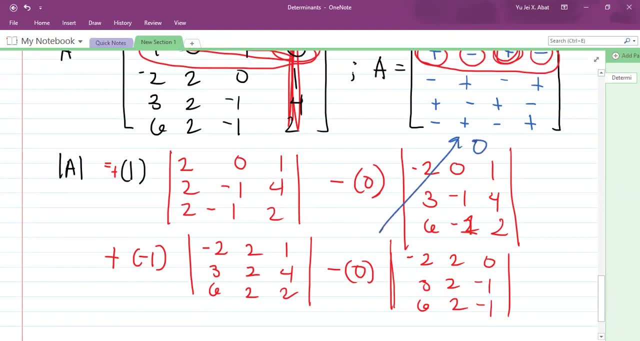 So, ayan yung magiging determinant ng buong four by four. So, kaya lang, para mapadali yung buhay natin, we can cancel this out. Ito, wala na to. Kasi kahit kunin ko yung determinant nito, imumultiply ko sa zero, zero pa rin. 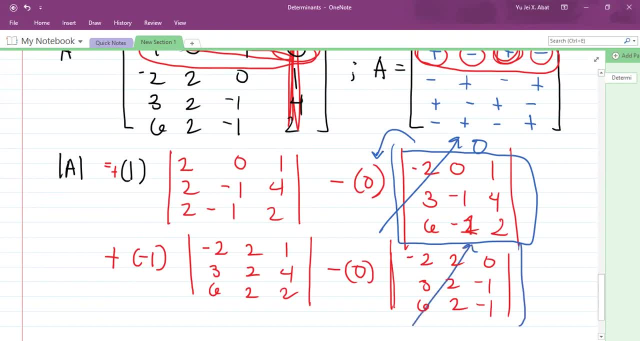 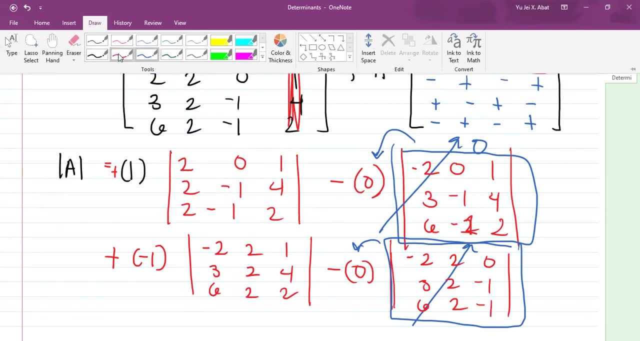 Ito, canceled out na rin to. Kasi kahit kunin ko yung determinant nito, pag minultiply ko sa zero, zero rin. So, ang matitira lang is yung dalawa. Kaya as much as possible, pag may maraming zero sa rows or columns, yun yung piliin ninyo. Mas madali yan. 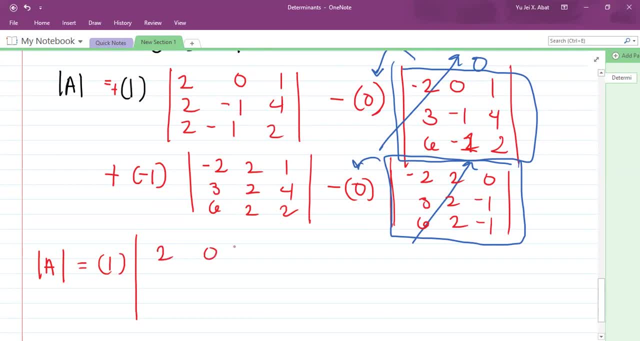 So, one times the... Determinant of two zero one, two negative one four, two negative one two. 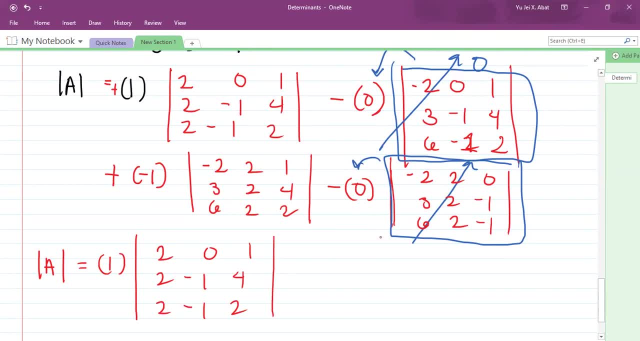 A plus, or pwede nga minus na eh, diba? So, pero sige, lagay pa rin natin. Okay. 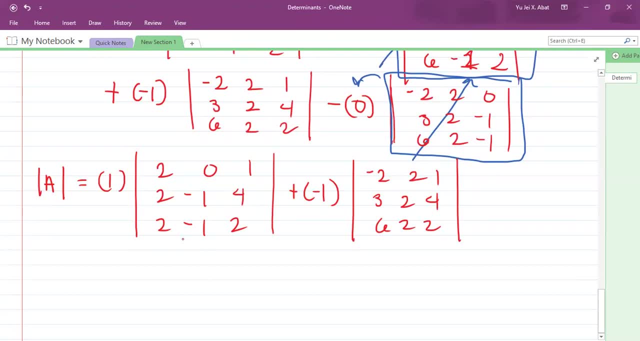 So, gagawin natin, kukunin natin yung determinant nito. So, let's say ito yung A1. Kunin natin determinant. So, determinant muna ng A1. 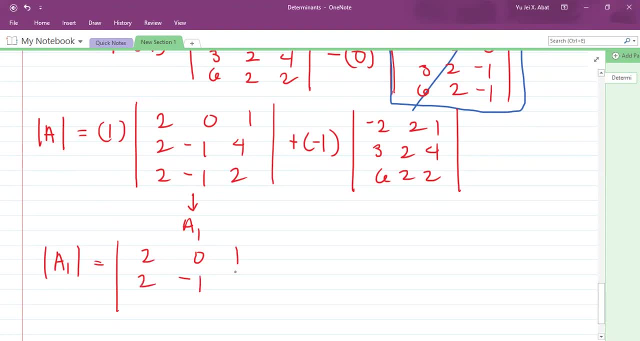 So, that's two zero one, two negative one four, two negative one two. Copy the first two columns. Two, two, two. Oy. Tama ba to? Two, two, two talaga siya. Oo nga. Two, two, two siya lahat. Okay. Let's see what will happen. 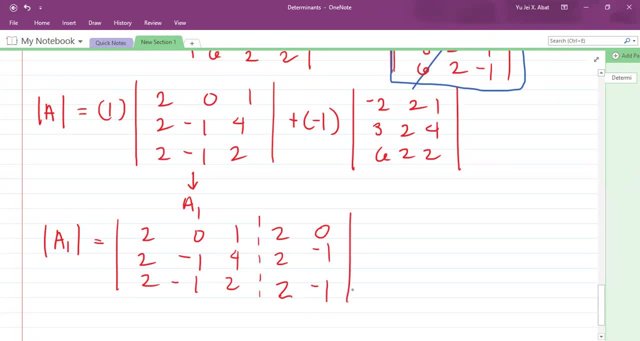 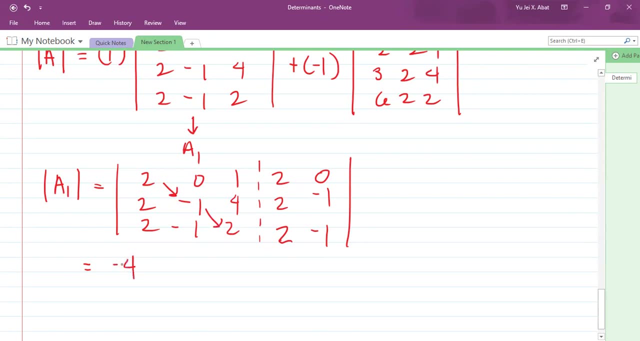 Two, two, two, zero, negative one, negative one. Okay. Kunin determinant. Determinant. So, two times... Two times negative one, it's negative two times two, negative four. Diniretso ko na. Plus zero to. Okay. 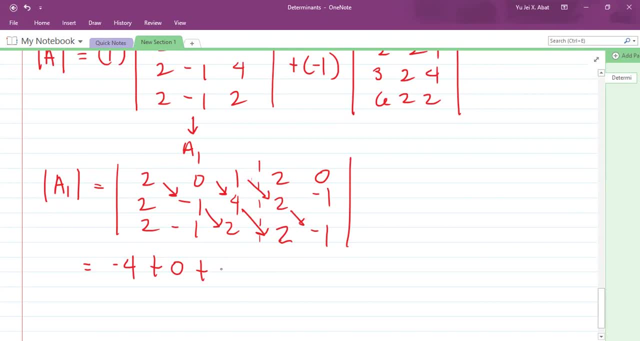 Plus one times two is two. Two times negative one is negative two. Minus the other diagonals. 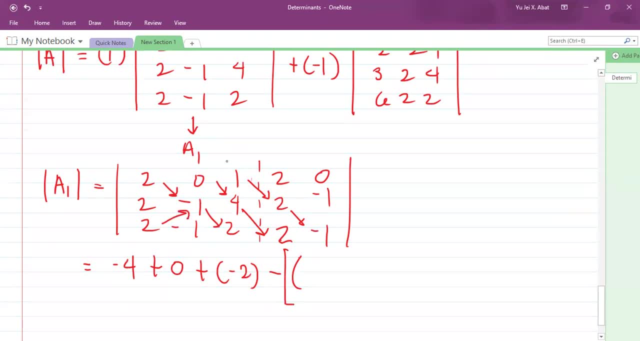 Two times negative one, it's negative two times one. So, negative two to. Plus. Okay. Okay. Plus. 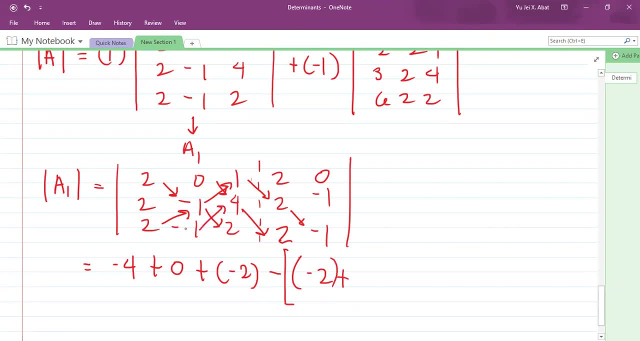 We have negative one times four. Ito yun. Negative one times four. 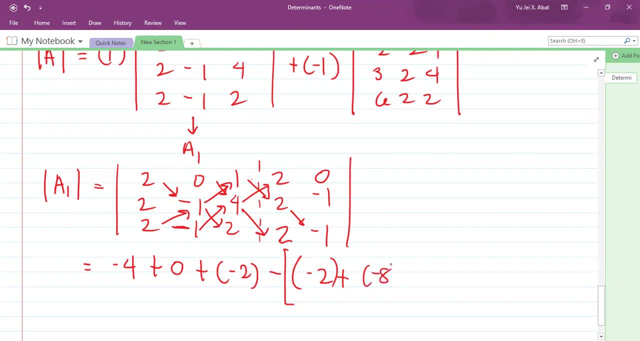 It's negative four times two. So, negative eight. Okay. 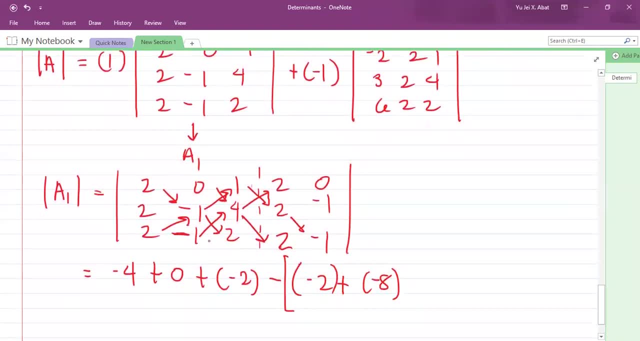 And then we have one for two. Two times two times zero would be plus zero. Correct ako na guys ha. Okay lang. Kasunod naman. Okay lang po siya. So, ganun lang din yun. 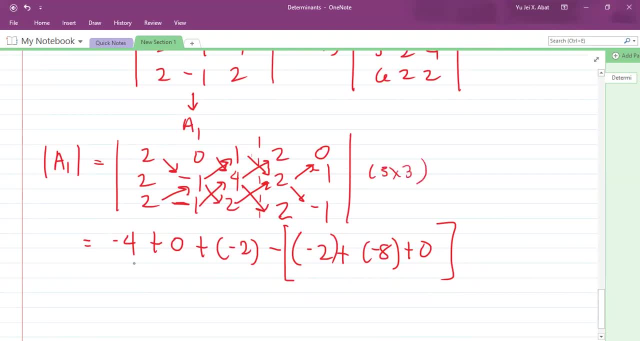 Yung three by three. Kung paano natin tinree by three. Ito. Inanok ko na lang. Kinuha ko na lahat ng product. Hindi ko na ina isa-isa. 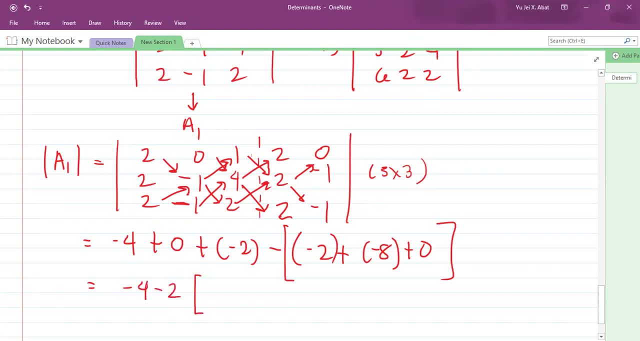 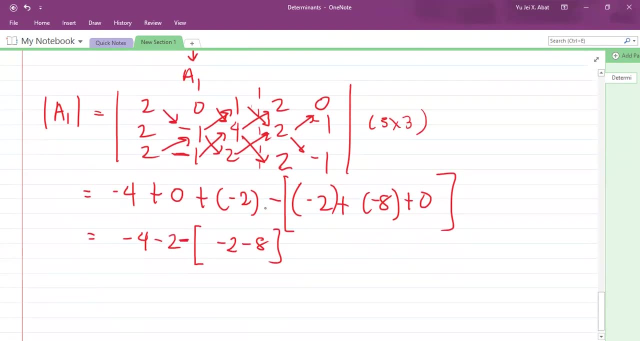 So, you have negative four minus two. Tapos meron ka pa ditong negative two minus eight. No? So, may minus ka pa dito. Because of this. Okay. So, negative four minus two. Negative six minus. Ito, negative ten. Distribute the negative signs. Negative six. Plus. We have ten. Which is four. Okay? So, ibig sabihin. This would be four. One times four. One times the determinant of this. Meron pa tayong isang determinant. Let's say ito yung A2. Kunin natin yung determinant niyan. 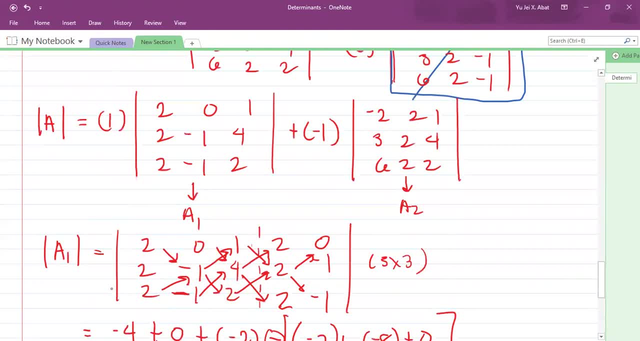 So, yung A2 would be negative two to one. So, negative two to one. 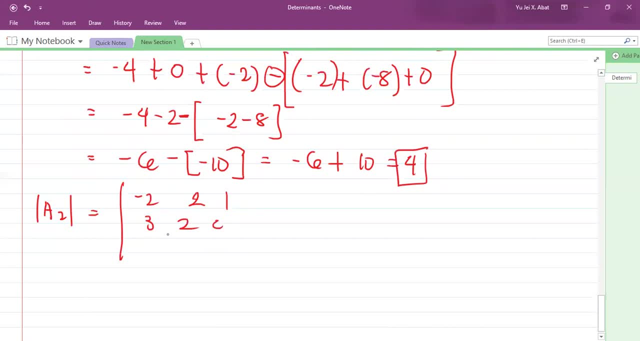 Three, two, four, six, two, two. Three, two, four, six, two, two. Okay? Copy the first two. Columns. Columns. Yan. Then, sige, rektan natin. Yan, no? 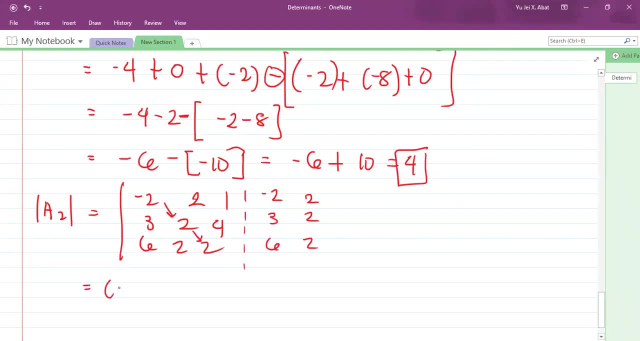 Four times negative two. It's negative eight. Plus. Two times four times six. Eight times six, eight, sixteen, forty-eight. Yan. Tama ba? Forty-eight. 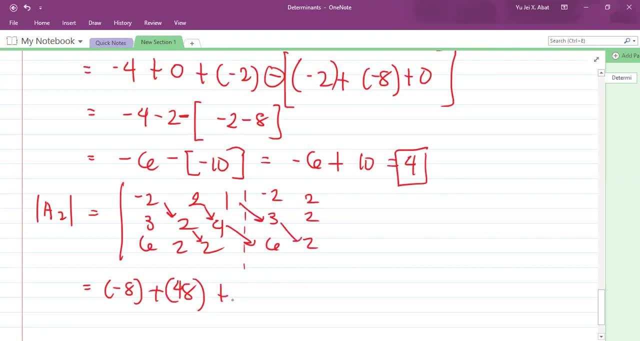 Then, plus. You have one times three is three. Times two is six. 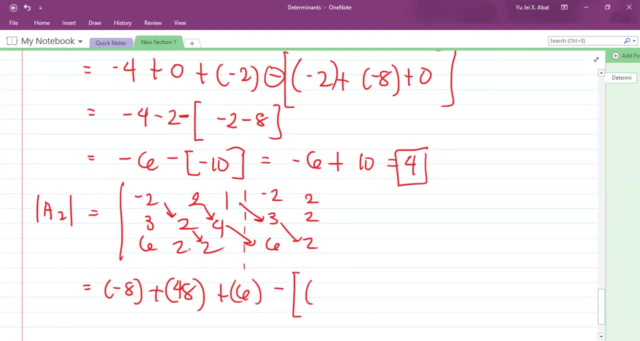 Minus the other diagonals na. Six times two is twelve. Times one is twelve. Plus two times four. Hindi pala yan. Hindi pala yan. Sorry. Six, diba? Six pa ganito. Then, ito. Two times four times negative two. Two times three times two. Ayan. So, four, twelve. Plus twelve. Kunin natin. Negative eight plus forty-eight. It's forty plus six. Forty-six to. Yan. 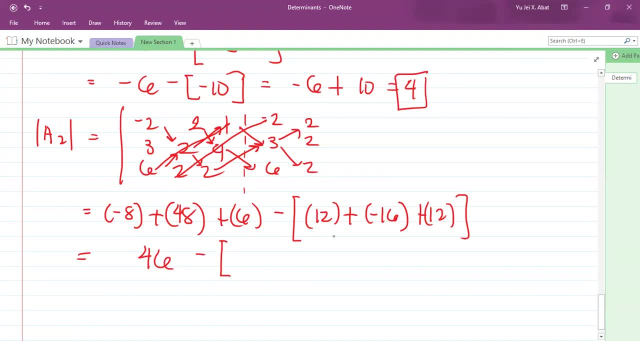 Minus, you have twenty-four minus sixteen. That is eight, no? Eight. So, meron ka forty-six minus eight. That's thirty-eight. Tama ba? Yan. Thirty-eight. 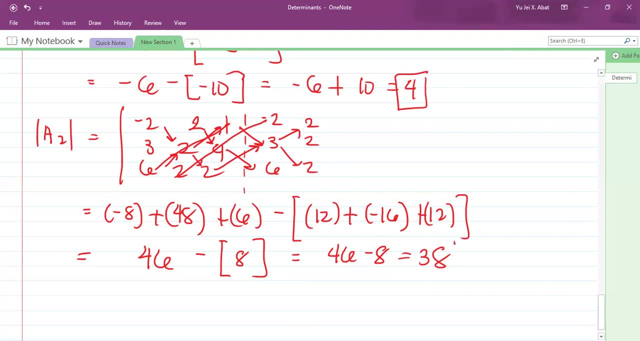 So, anong gagawin? Yung determinant ng A, yun na yun. So, diba? Meron kang cofactor na one. Ito. 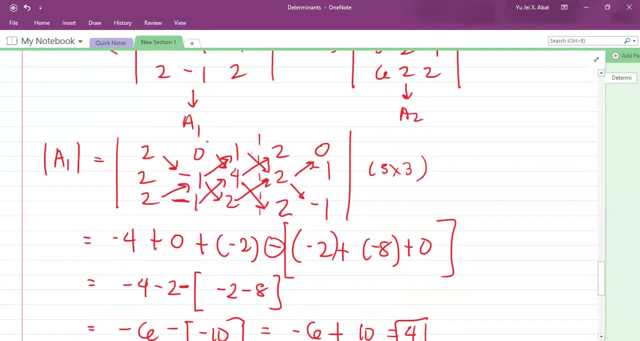 So, we have one times. Yung nakuha natin na determinant ng A sub one na to. Determinant nito. That is four. Okay? And then, we have plus negative one. Diba? 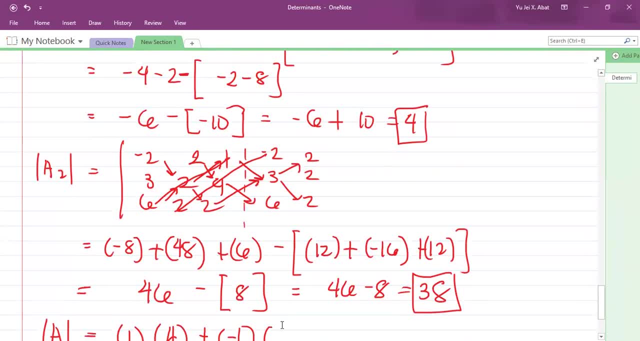 Plus the negative one. Negative one multiplied by the determinant nung pangalawa. Ito yung A2 natin. Yan. Which is sinolg natin. Naging ano siya? Thirty-eight. Yan. 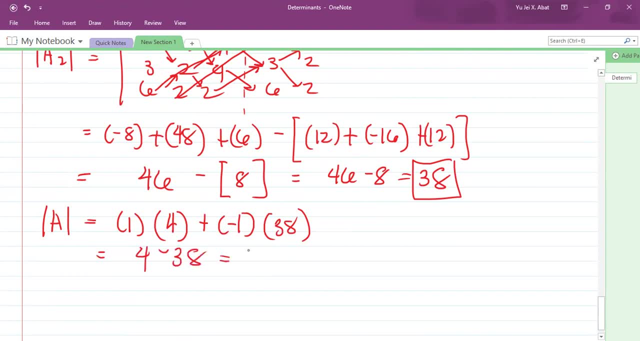 Four minus thirty-eight. So, negative thirty-four. Question. 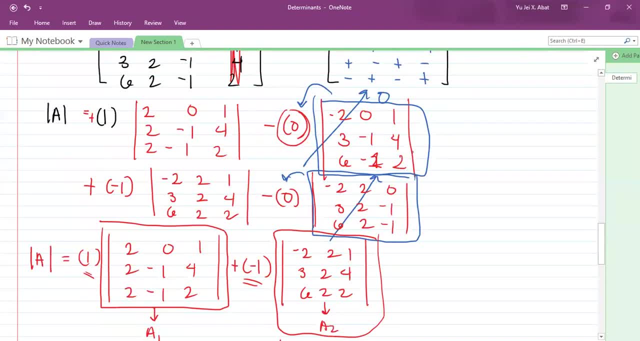 So, kung hindi zero ito, nag-determinant ka pa ulit. Ito. Sinama mo ito at ito. Pero, since zero na yan, any number multiplied by zero will be zero. Question, guys. 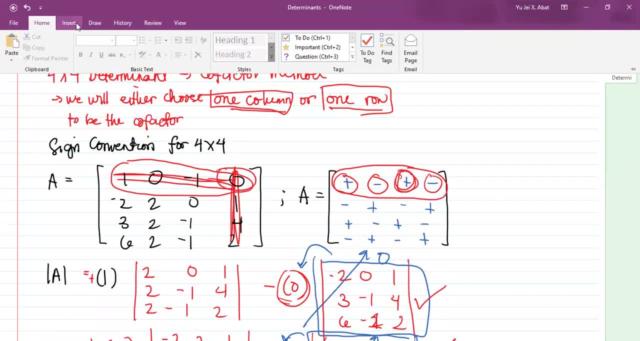 So, ito. Ito yung papagawa ko sa inyo, no? So, mapapractice. So, mapapractice na yung lahat ng determinants ninyo. 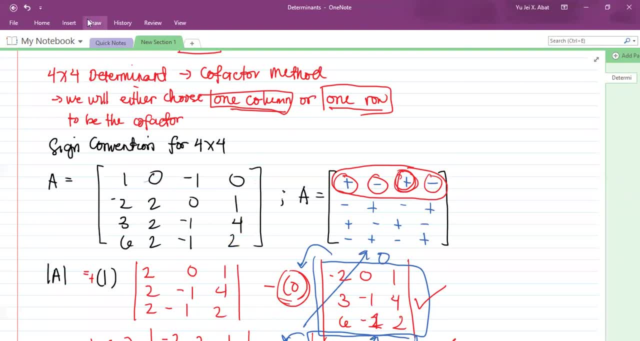 So, ngayon, your problem set would be... Okay. 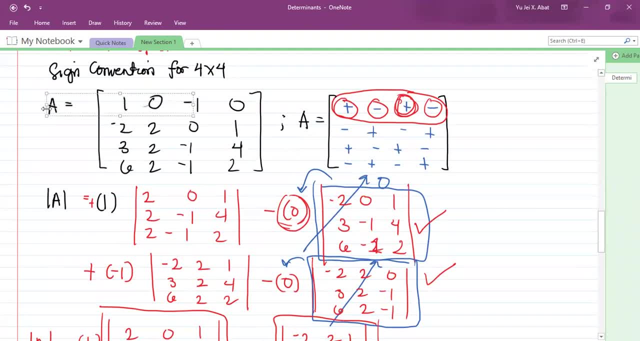 Kokopihin ko lang ito. Ay, di na. Bago na lang. 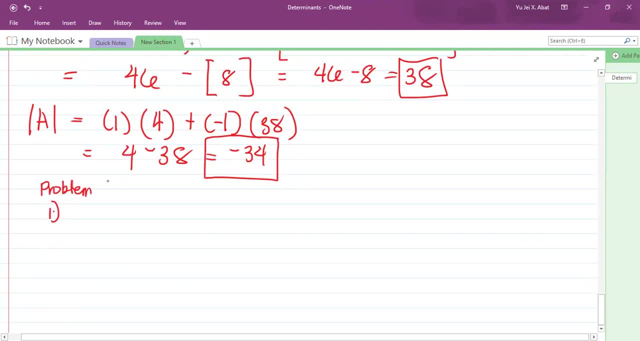 So, problem set tayo. Find the determinant lang naman. Okay? Yun lang. With your complete solution. So, find the determinant for matrix A. 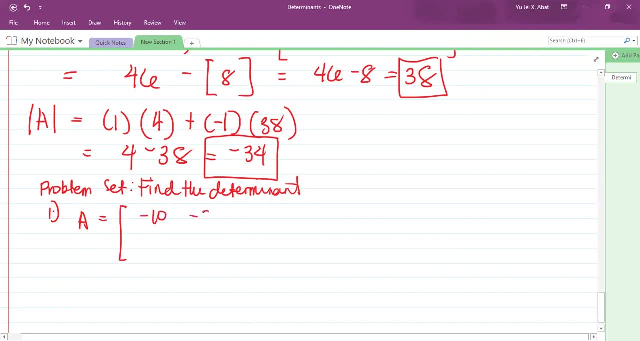 We have negative ten, negative two, negative five, and one. That's for matrix A. For matrix B, we have a three by three. 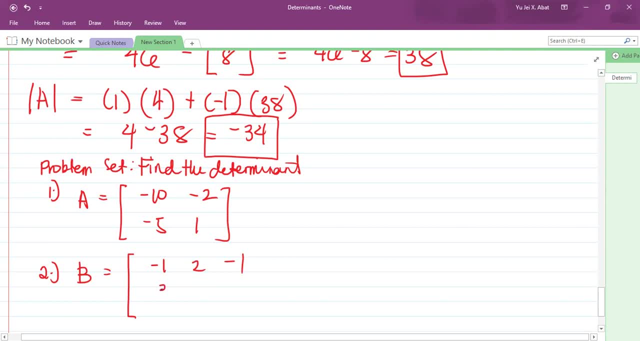 Negative one, two, negative one, six, three, six, nine. Twelve, negative ten, and negative five. 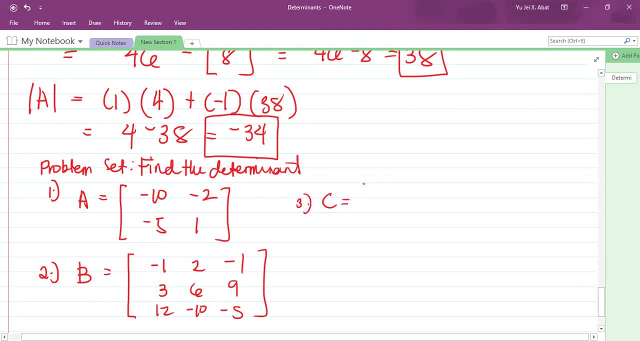 And for number three, okay, matrix C. That is a four by four. 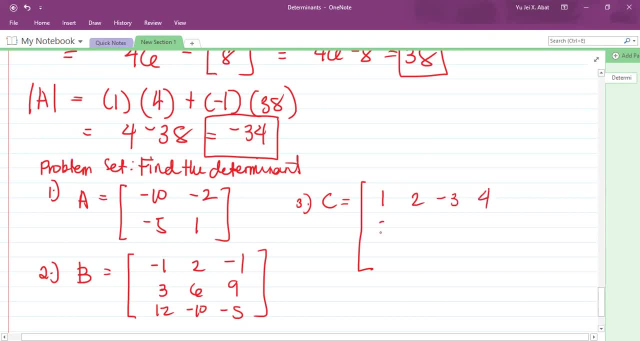 One, two, negative three, and four. Six, seven, negative five, negative ten, negative twenty. 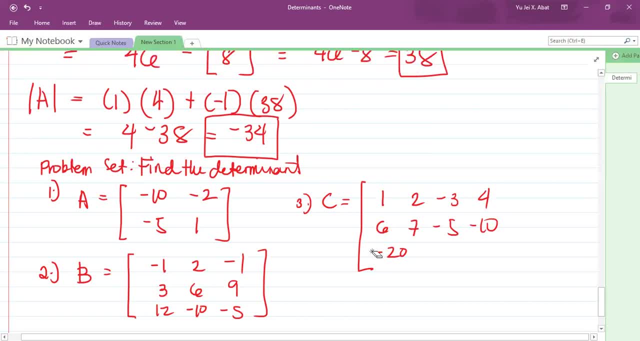 Wait lang. Medyo hindi ayos yung aking pagkakalagay. Para align sila. 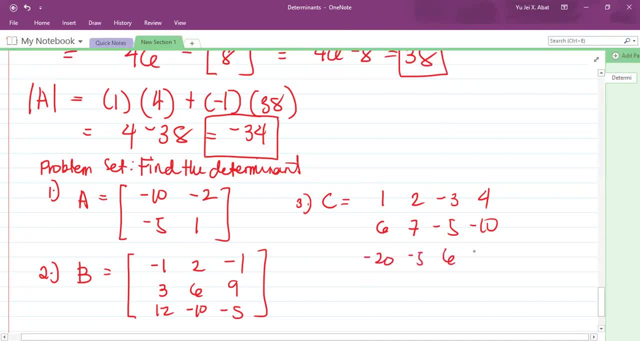 Negative twenty. Negative twenty, negative five, six, seven, eight, nine, negative ten, and negative two. 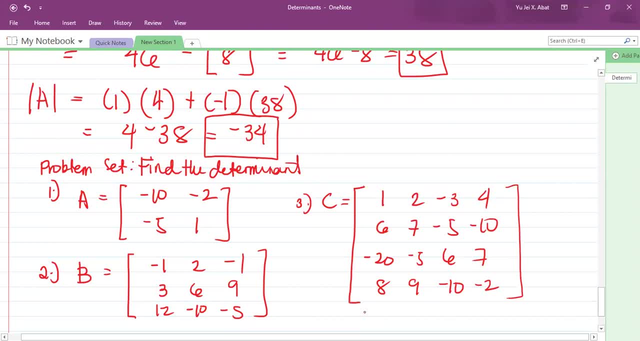 So, find the determinant. Now, dito, use cofactor using the sign convention. Kahit anong piliin nyo dyan. Kahit anong piliin nyo dyan. 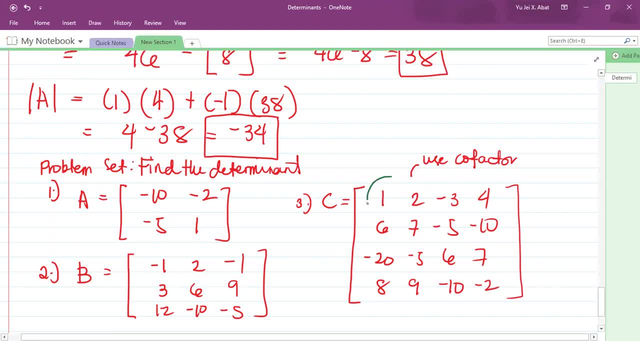 Kahit ito yung piliin ninyo. Pwedeng ito. Okay? Okay? 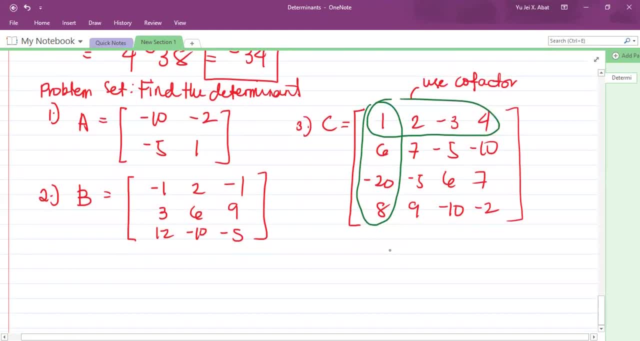 So, basta pagpiliin ninyo, follow the sign convention. Yung magiging sign convention, again, would be positive, negative, positive, negative. Negative, positive, negative, positive. Okay? 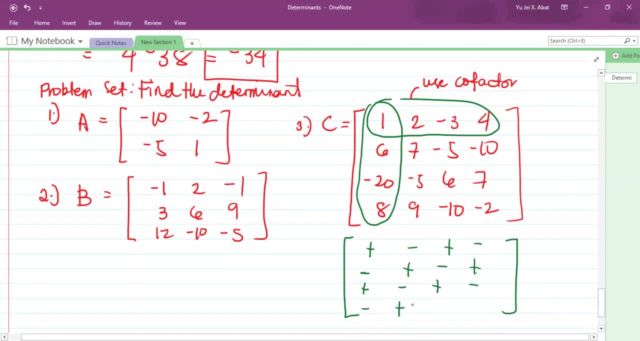 And then positive, negative, positive, negative, negative, positive, negative, positive. Yan ang sign convention. 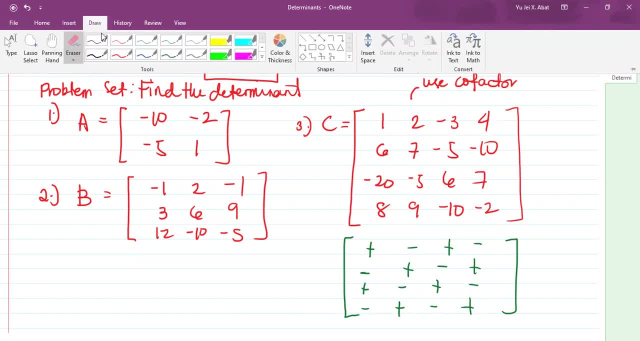 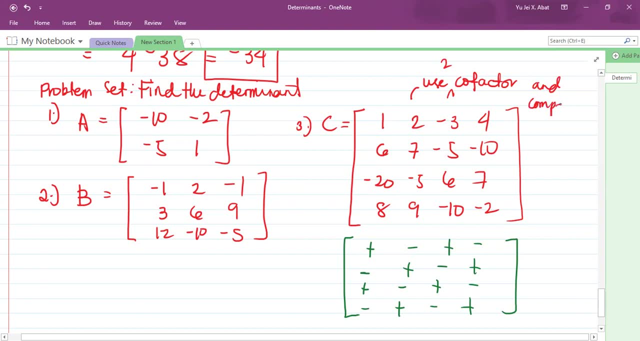 Tapos, ang requirement ko pala dito is that use two cofactor and compare the answer. Siyempre, kapag gumamit ka ng dalawang cofactor, kunwari, ito yung unang ginamit mo, may other solution dyan. Tapos, yung next, ito na ginamit mo, may isa pang solution dyan. So, pag parehas ng sagot, tama yun. Kasi dapat equal lang. So, bali sa number three, parang meron kang 3.1 and 3.2. The first cofactor, nakuha mo yung determinant. And the second cofactor, yung nakuha mo yung pangalawang determinant by choosing any column or row here. 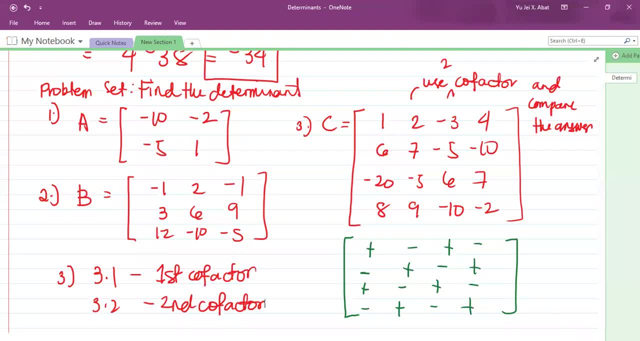 Picturean nyo lang. Problem set natin yan. Picture, screenshot. Okay? Okay? So, you can just picture what. So, yan. 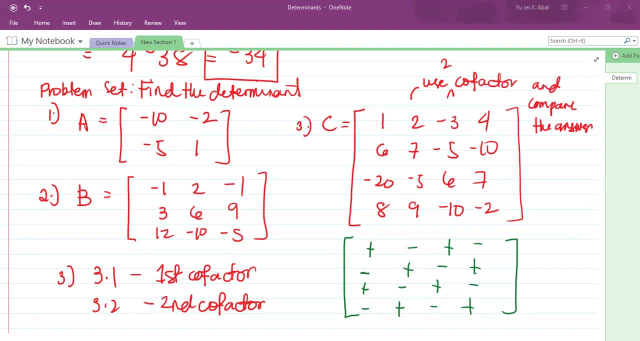 Submission yan next week. Next week, Thursday. Sir, tanong ko lang po. Yes? Yung lab po, ilan po yung tasa? Ha? Yung laboratory. Ay, sa kabila pala. Laboratory. Pala. Sa kabila pala. 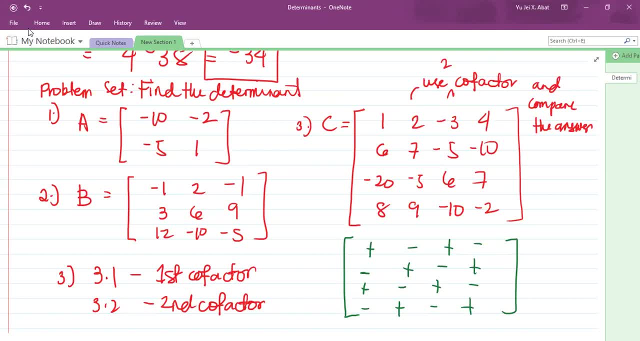 Hmm. Okay. Questions. Wala naman. Wala na po, sir. 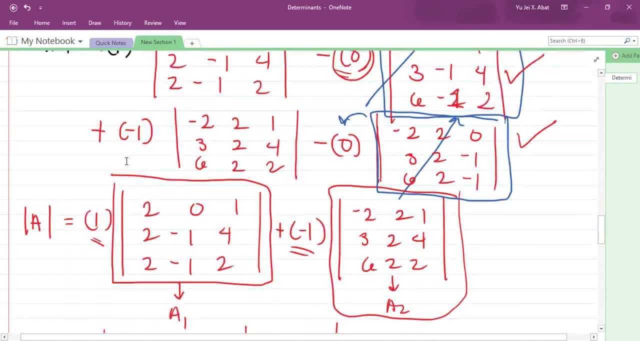 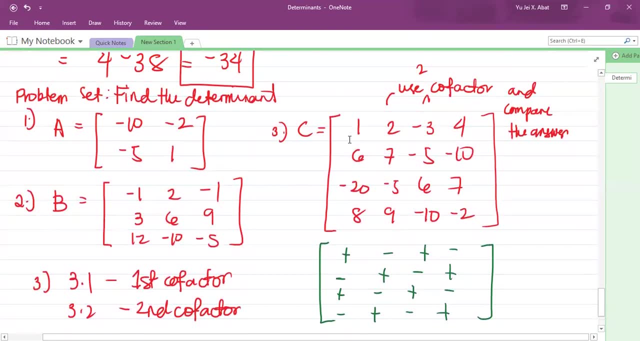 So, malinaw yun, guys. So, pag alam nyo na yung 3x3 sign convention, madali na lang para sa inyo. Takip-takip lang. Kapag nakakuha na kayo ng isang cofactor, takpan nyo lang. Tapos yung matrix na matitira, yun yung kukunan nyo ng determinant. So, may questions pa ba? Questions? Clarifications? Wala naman. Wala naman po. Okay. So, yun lang guys. Stop ko muna.